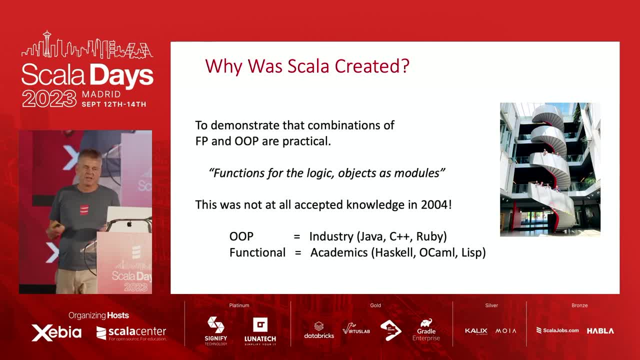 slides and in the talk. So let's start with the beginning. Why was Scala created? Well, when was it created? That's a long time ago, It's in 2004.. And the reason why was? I wanted to demonstrate that combinations of functional and object. 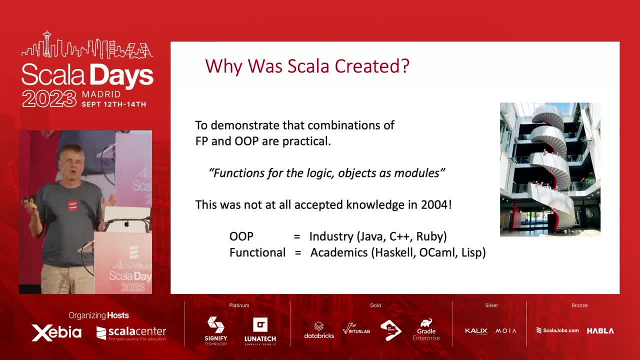 oriented programming could be practical. There was a lot around during that time. Object oriented programming was the industry standard, undisputed And functional was essentially all academics In industry. there was no traction whatsoever. But there were a lot of people who thought, well, maybe we can take the best of both or combine the two. And I thought: 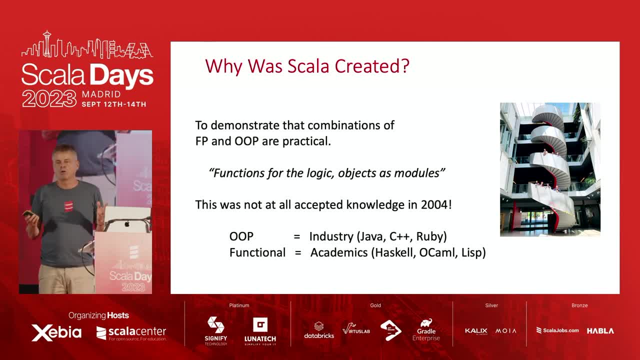 I had some idea how to do it and worked more on essentially small languages, calculi, things like that, And until at some point I thought, well, I think this could actually work. Now we have to show that it can actually be practical, And initially it was essentially just intended. 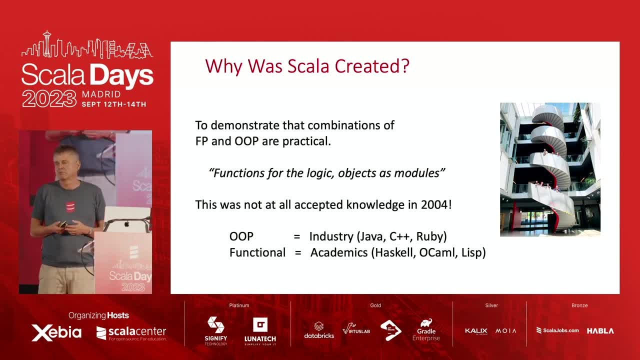 as a demonstrator to show that you can write useful programs with that. In the first years we got one or two users, probably not many more than that, And then suddenly it exploded in 2008 that companies like Twitter picked it up and Foursquare and others- Twitter. 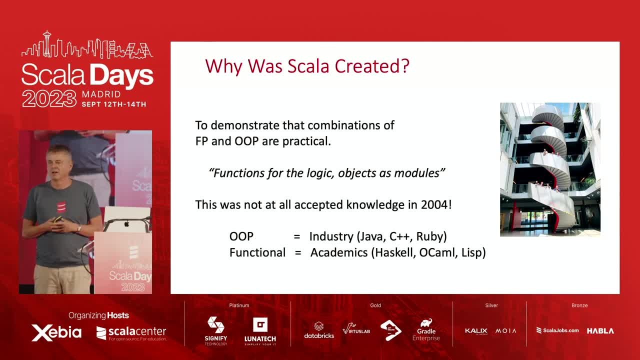 you must know at the time was a company of 25 people, including ops, So it was a startup, basically, And they were doing Ruby and having too many fail wells, too many crashes. So the investors told them: do something serious, go on the JVM. But they were language enthusiasts. 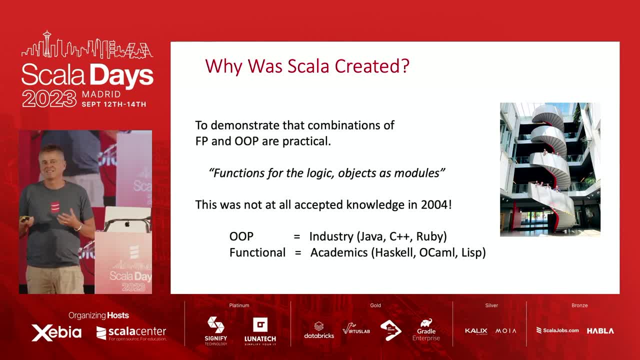 and say: well, we want essentially a language that lets us express ourselves better. And well, there was this. There's this new kid on the block, which at the time was Scala, And it runs on the JVM, So they picked that, And the rest is history. 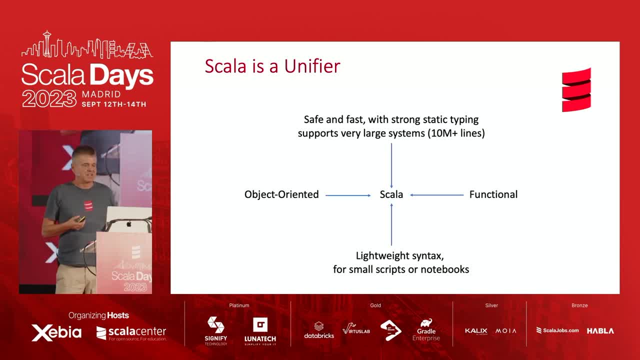 So the early slides, I always had essentially this slide to say: Scala really is a unifier in many dimensions. In particular, it's a unifier between object-oriented and functional. As we know, it's not just essentially two languages side by side with one set of constructs. 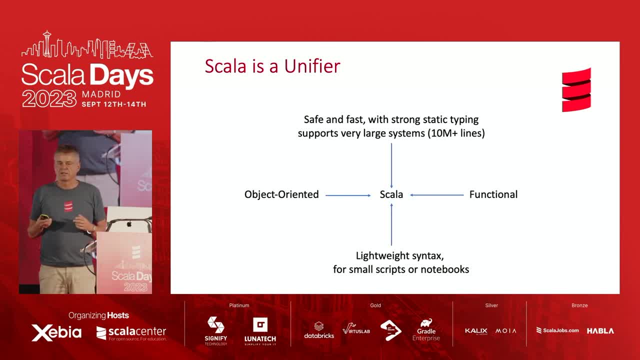 geared towards functional and the others towards object-oriented. They're one and the same. So a function is an object and an object is a function. It's really one and the same things that you can smoothly use everything from one side on the other side to a degree. 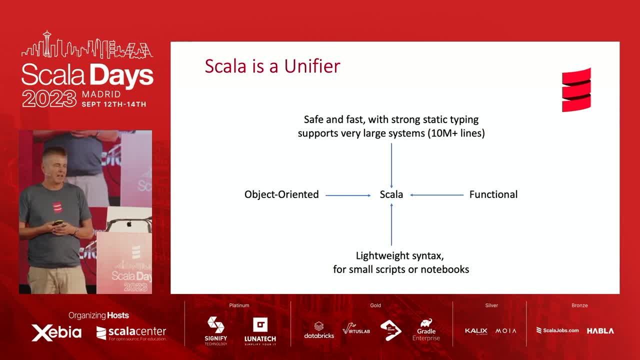 where you don't notice that there's a difference, and one should really invent a new paradigm for that. functional object-oriented is still two words. We would need something shorter than that, And with that. the other claim was that we get a very scalable language, that 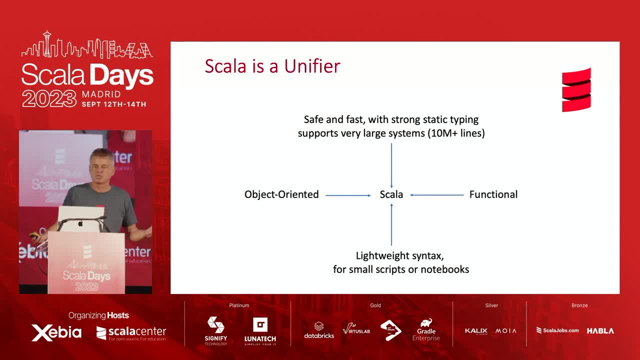 can go from Light white syntax for small scripts and notebooks to very, very large systems, And that's also true. I mean Scala is a very good language for scripting, for using it in the REPL, for exploring, for teaching programming, all these things, And at the same time it 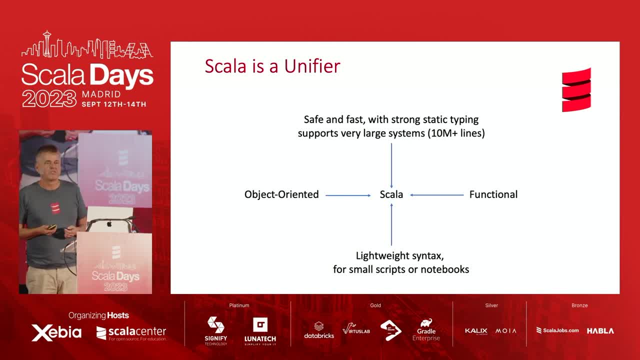 is a workhorse for systems of 10 million lines of code and more, And the interesting thing is that it achieved all that with one set of constructs. It's objects from the REPL to these large systems And there's nothing bigger than that for programming in the very large or things like. 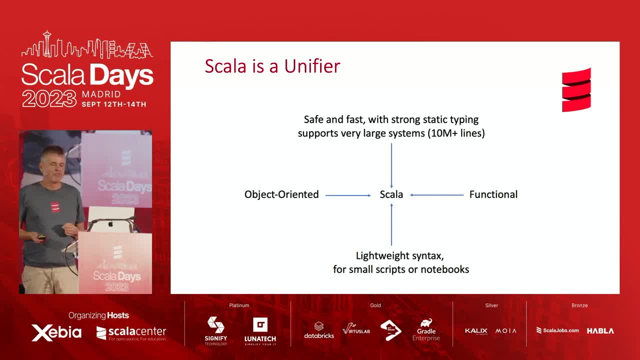 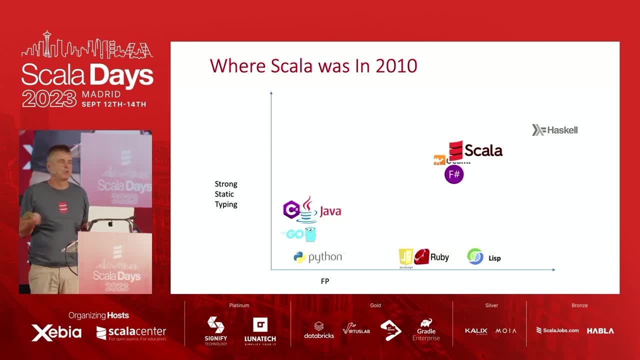 that The claim at the time was: that's possible And I think we have proven by and large that it is So. then Scala became popular. A user community formed quite enthusiastic, And at the time, why did that happen? I think it happened because Scala had a fairly privileged spot. here you 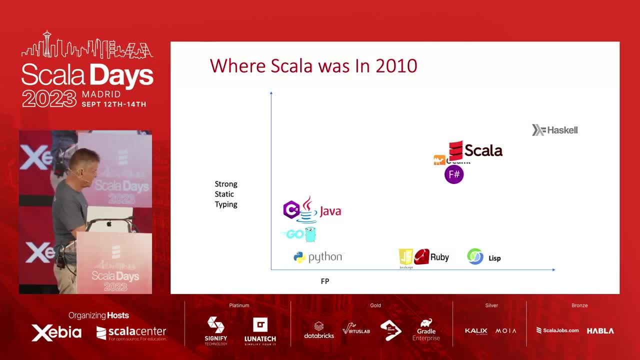 see on the right And you see whether the laser here works. not really Okay, But you see, you see it Probably okay, But you see it, You see it big enough. So it's a language that is, the lower access is functional And the upper axis years stronger. static typing. 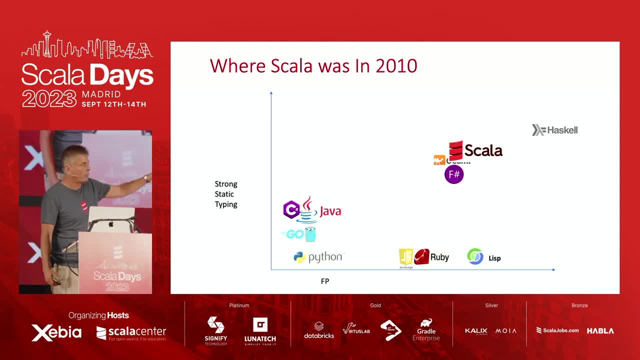 it's a language that is goes quite, quite a long way in both without being maximalist, so it's not a hundred percent functional. It's a language that essentially prefers functional but does it force you to be the 100% pure, And the same holds with type systems. So it's a language that has strong static typing. 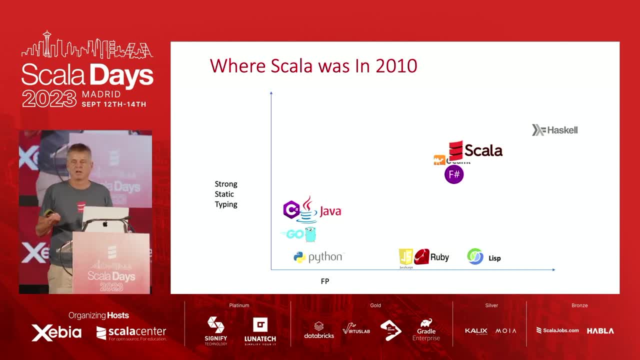 support. But if you want to use it in a loser fashion with essentially more patterns coming from dynamically typed languages, that's also possible. So it really sits in there. And there were a couple of other languages. OCaml was there already. F-sharp came later, But it had sort of 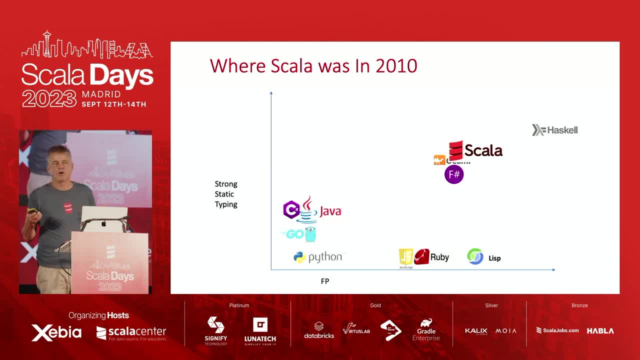 the field more or less to itself, And that essentially caused a lot of people to pick it up and do great stuff with it. from the Twitter stack to Akka to Spark Flink- Lots of really cool software was written in Scala. And it was written in Scala because, essentially, people saw 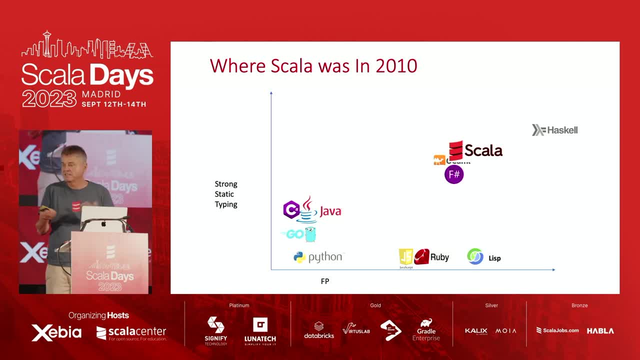 that here was a language that lets us express these things easily and quickly. Okay, So that was 2010,, a long time ago. What happened since? Well, what happened is that, basically all the other languages- they moved towards that Very direction, right, So they became more strong, stronger, typed, more types, A lot of the 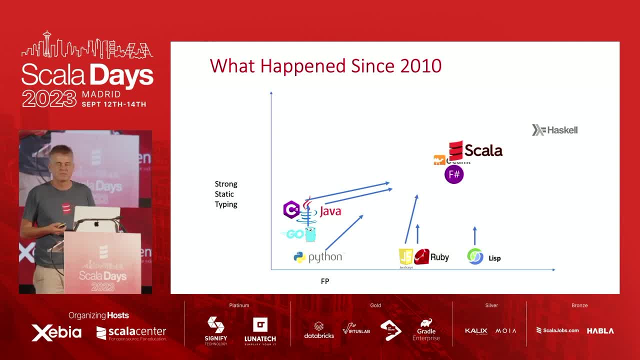 dynamically typed languages acquired optional type systems in the meantime, And they became, by and large, more functional. So the fact here is that- let's just see I'm missing a slide here. Okay, And what happened then in the end is that 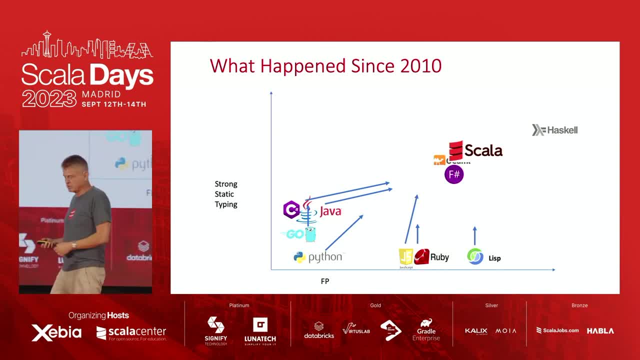 you. essentially, a lot of languages ended up much, much closer to Scala. not just the existing ones, which were around in 2010, but also a lot of new languages that came up since then. Whether you talk about Kotlin or Swift, or Rust or TypeScript. all of them are very much in that space and have 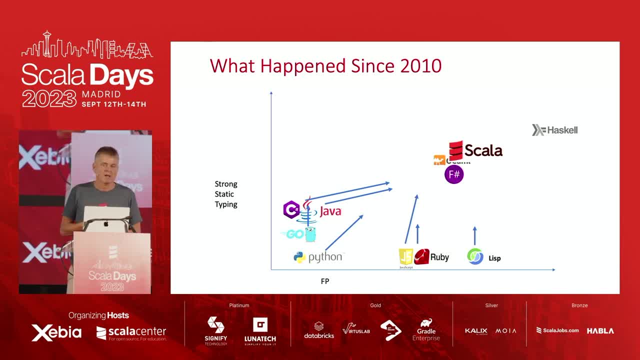 adopted quite a lot of features that Scala has pioneered. Now that you see all these, this language zoo, it's maybe not so apparent of what things Scala is going to be able to do in the future. I think it's going to be a lot more. 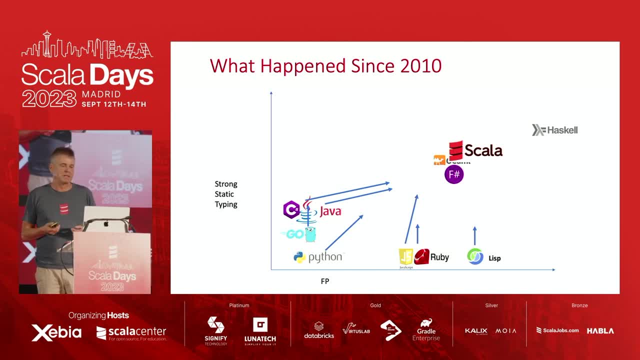 common. So actually Scala was the one that pioneered them. That means it introduced them, or at least it made them popular. Maybe sometimes they were already introduced before. So I'll just give you a list of some features that were essentially Scala firsts. So first one is X. 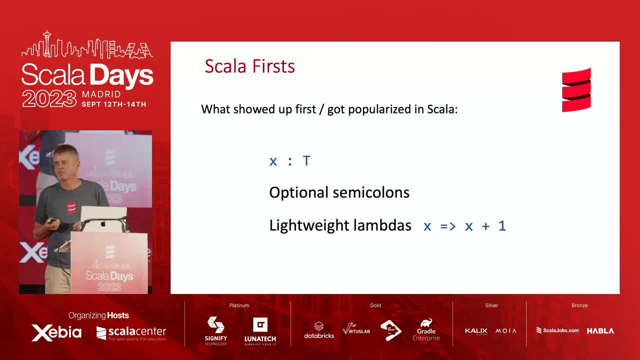 colon T, I say, well, that's a Swiss notation, right, It was already in Pascal and now it's in Scala and things like that. True, And so it means it's a lot older than Scala was. It probably was. 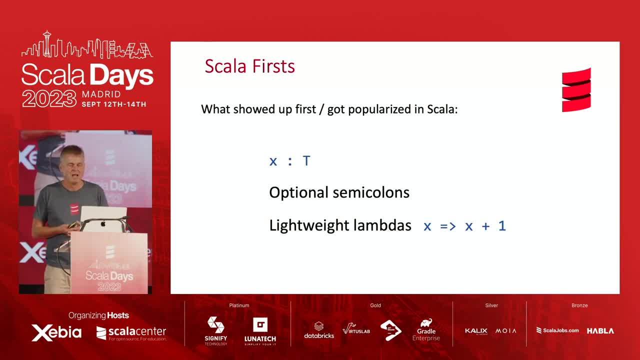 introduced by Pascal or one of the predecessors of Pascal, but in the time when Scala was introduced, 2004, that notation was essentially non-existent, so all the languages that used it had gone out of existence. there was still ML, but ML was essentially, like I said, an academic niche. 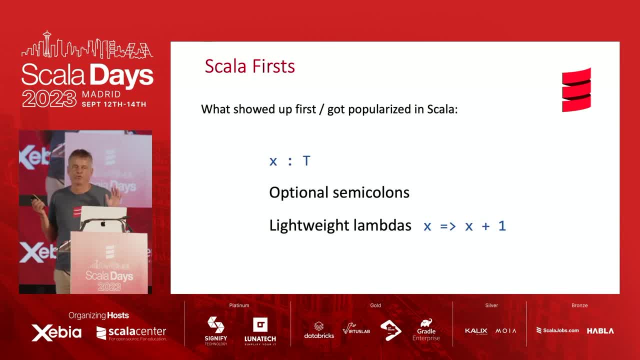 languages and that was essentially something that was completely different and when we introduced that there was a huge resistance. that's why I put it up first there. for many, many years people said: tell me, Martin, if you only had written tx, we would take your language seriously, but x, colon t, 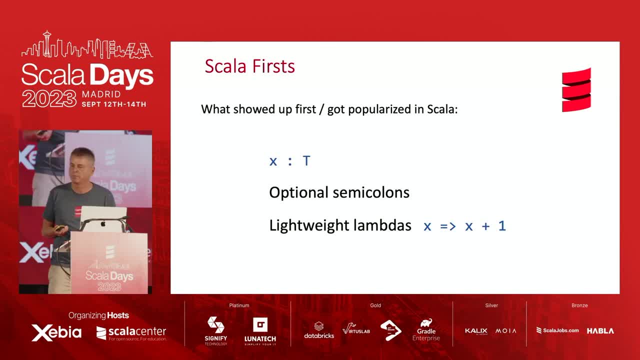 uh, forget about it, it's just. it's just too much of a of a jump. uh, it's too much of a of a change. and now, of course, well, what happens? all the new languages use x, colon, t or xt in the case of go, and almost nobody uses the, the opposite convention, anymore. another thing: to stay with syntax optional. 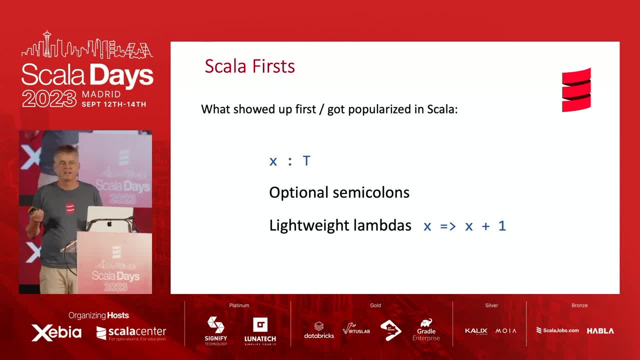 semicolons is something that existed in JavaScript before, but it never worked very well. in Scala, we essentially invented the rules to make it work solid, so nobody in Scala land is missing semicolon or is writing them. it's been a long time that I've seen code that used semicolons. 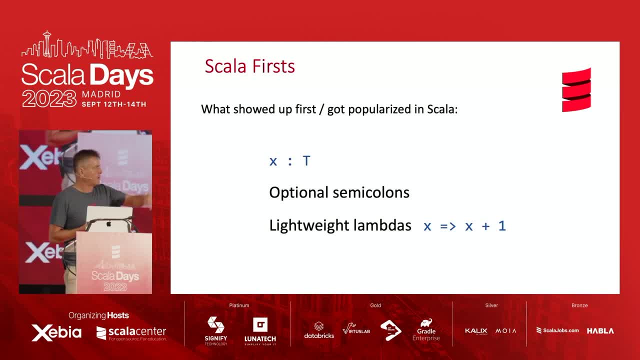 light. white lambdas is another thing. so this x arrow, x plus one syntax was, as far as I know, invented by Scala and has been copied by a lot of other languages since. another thing that is very important is expression of the language orientation, that, so that Scala doesn't split, doesn't distinguish between statements and 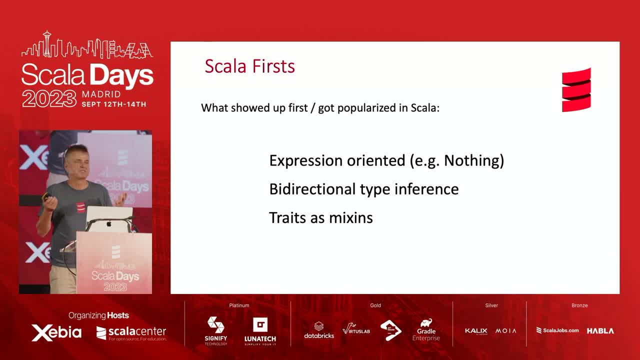 expressions and if you it's for, for us it's completely natural. of course, everything is an expression. of course I can have an if, then else that can return values. of course I get one of these branches can be a throw that throws an exception. all of that is completely natural. but 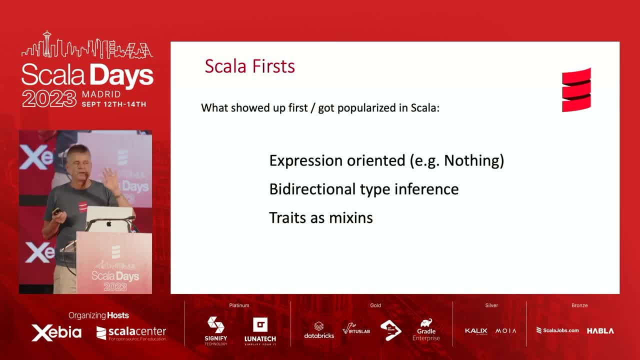 it isn't. it wasn't before. there was a world of expressions or a world of statements and, for instance, I had a nice talk by Andre Breslau, the original inventor of Kotlin, or one of the original inventors, who said he talked with Anders Halsberg, the inventor of c sharp and later on typescript, and said: well, it's really cool. 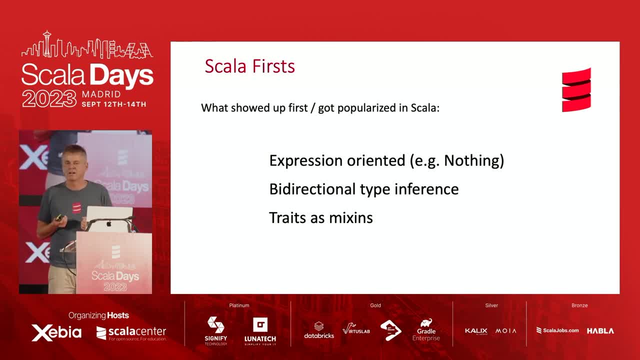 this throws in in in Scala can be an expression that that's really nice, it should be an expression. and Anders said, yeah, but what? what should its type be? it can't be unit. if it's a type of an expression- and that was it for Anders- then. so it turns out that if you take expression orientation, 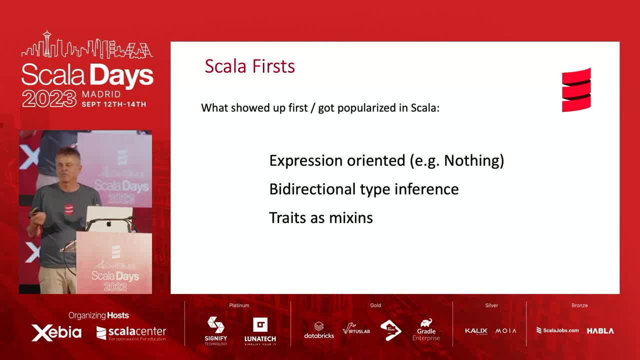 seriously, then you have to. you have to invent the nothing type, you have to invent bottom, and so there's a lot of other things that seem random in Scala, maybe at first, when you get get around them at first, but which have a reason like that: for instance, nothing for expression, orientation, other things that we are now quite used to, and 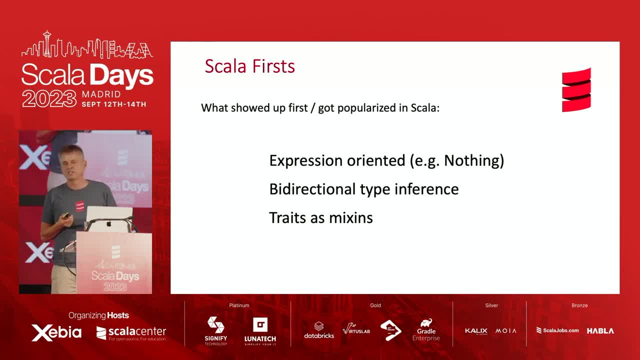 that I believe worked really well are the, the form of type inference, which is sort of not global, it's not a hundred percent, but it works actually pretty well in practice and it reinforces good habits that you should declare your parameters, and that's what we're going to talk about in a few minutes. 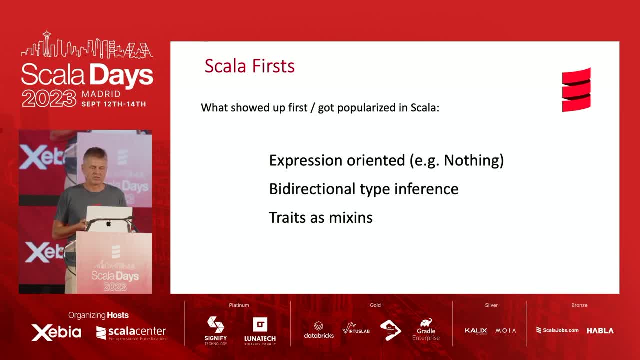 and that's what we're going to talk about in a few minutes of functions and and for public functions also, the result types. the idea of having traits as mixins is another thing that essentially gives you flexible composition of, of, of aspects, of components, and I think there also- Scala was the first- 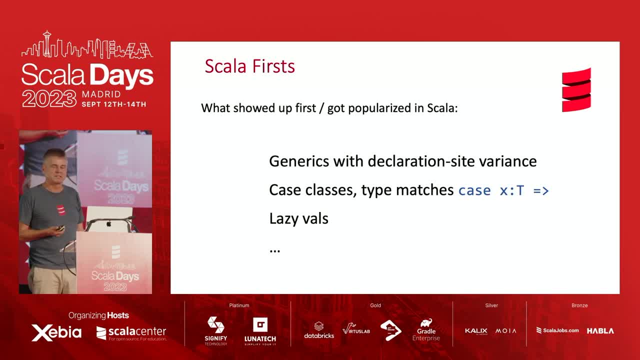 further things are generics with declaration side variants, the kind of pattern matching we do with case classes and these flexible patterns where you don't just have these deconstructors but also case these, these things. they were all first in Scala, lazy valves, and the list goes on and on. okay, so 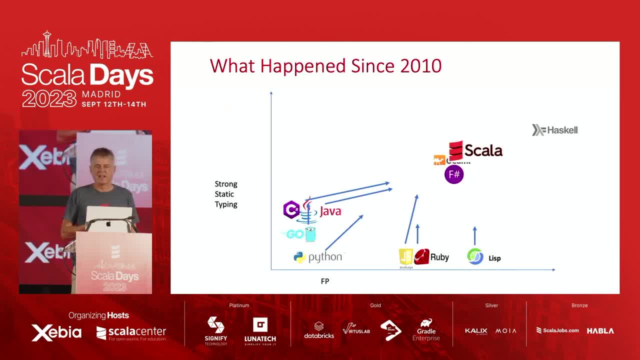 what happened since 2010 was, like I said, there were all these languages moving and now there comes the other slide, so now they're much closer to Scala, and they're all these other languages as well. okay, well, I could say, well, I'm, I could, I could retire now and said: purpose achieved. 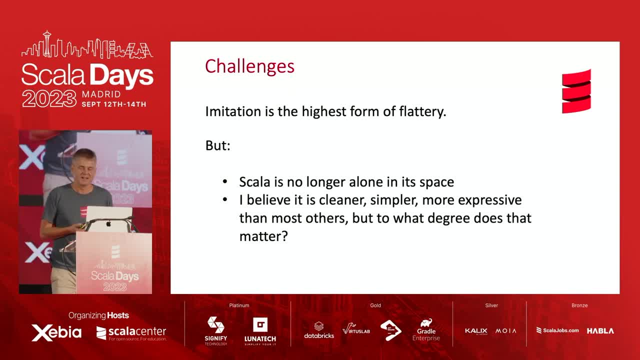 imitation is the highest form of flattery. right, but there are. I. I do do care about Scala, and there is a challenge that Scala now is had, no longer has the space for itself, it's no longer alone in the space. I like to believe that it's a cleaner, simpler 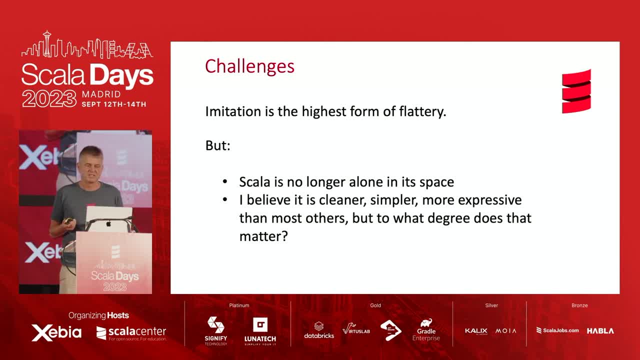 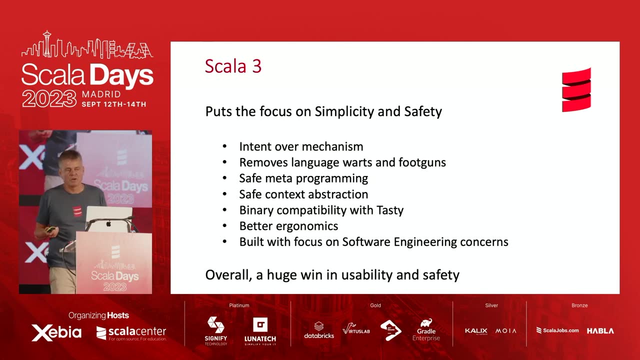 more expressive alternative to most of the other languages. but on the other hand, in industry, in, in the actual field out there, to what degree does cleanliness, simplicity, expressiveness really matter? well, what the? my reaction then was to say: well, we want to really make the other languages are catching up. let's make a big jump forward into the abyss. no, I'm joking. 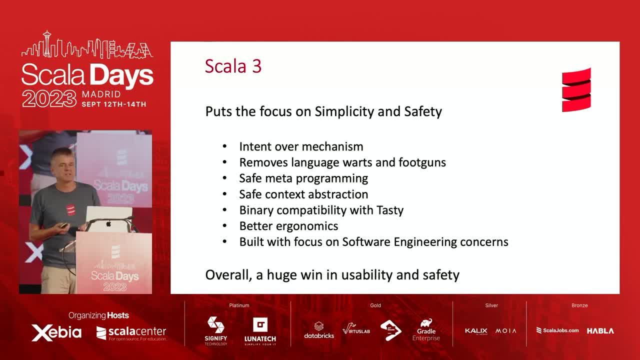 and that was Scala 3.. so Scala 3 was a reinvention of Scala. it says we are willing to break some things because we have the safety net of binary compatibility. that makes it work for us, and we want to put at the same time, the focus on simplicity and safety. that means sometimes in previously in 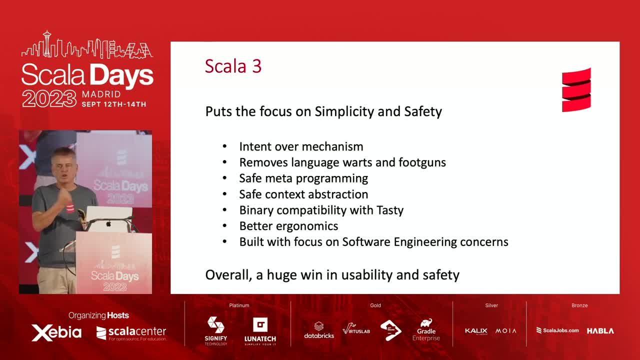 Scala we had very powerful mechanisms that could do lots of different things, but then when you read the programs it wasn't too apparent what, for instance, all your implicit constructions were supposed to achieve. so in Scala 3 we had this motto to say: we want to where it's possible. 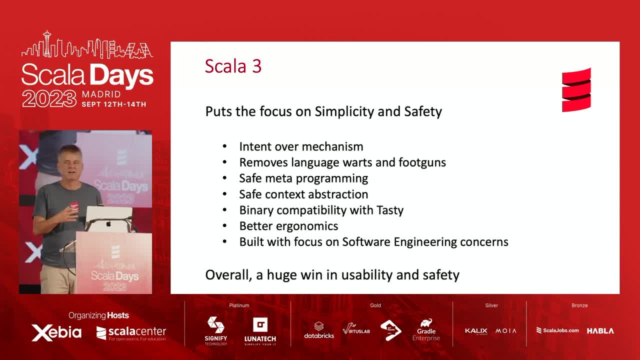 focus on intent over mechanism. we want to make it clearer what the intent of what your trying to achieve in your program is over the low level and very general mechanisms that that that are there. we worked hard to remove as many language wards and foot guns as we could. 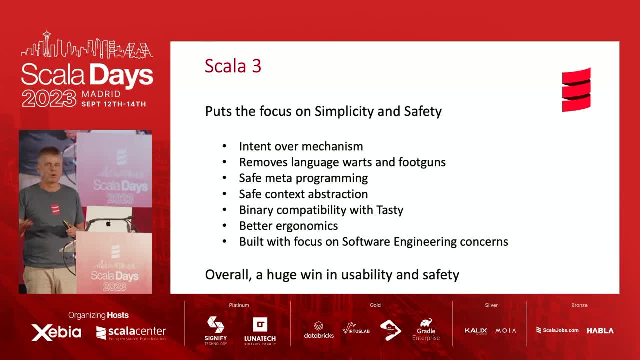 in particular there's now safe meta programming. that was probably the the biggest difficulty moving forward but also one of the biggest achievements: that we have meta programming that is independent of essentially some intricacies and and pitfalls of the actual compiler that runs meta programming now as a spec. it has safe foundations. the other thing is we have a much 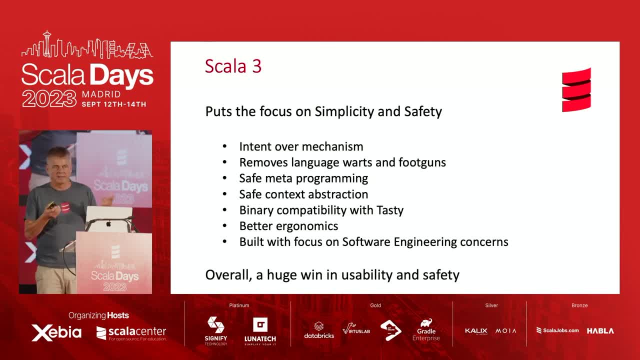 safer context abstraction. and the third one is binary compatibility is achieved with Tasty. so that's also a huge thing. that would be the times of where every so many years we had to sort of switch and go from 213 to 214, 215, and then everybody had to recompile with Tasty. those times 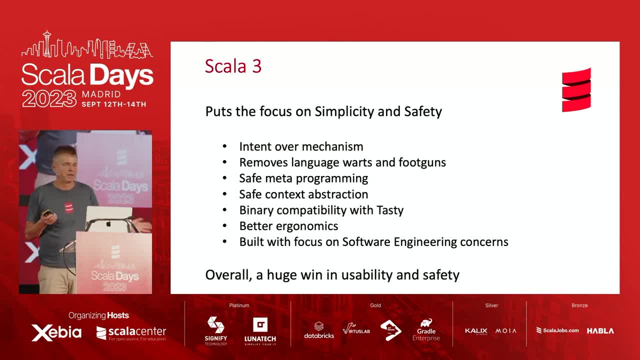 are over, so you don't need to do that anymore. it's back to normal. so that's one of the things that we want: to make sure that it's compatible forever. then also, we concentrated on better ergonomics and with a focus on software engineering concerns, because, unlike the green language designer, that 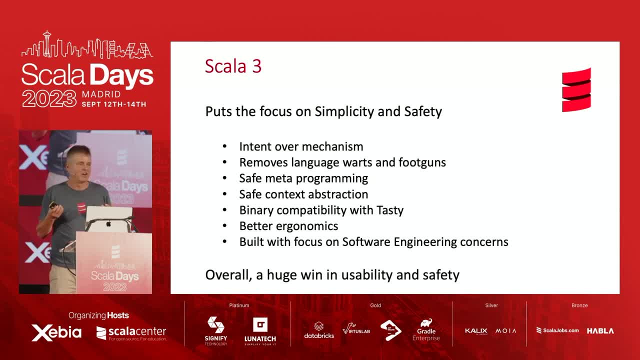 that I was 20 years ago. we have collectively learned, of course, a lot from the community how they applied Scala, what were difficulties and things like that. so it's a huge experience that all has flown into Scala 3 and I believe overall it's a huge win in usability. 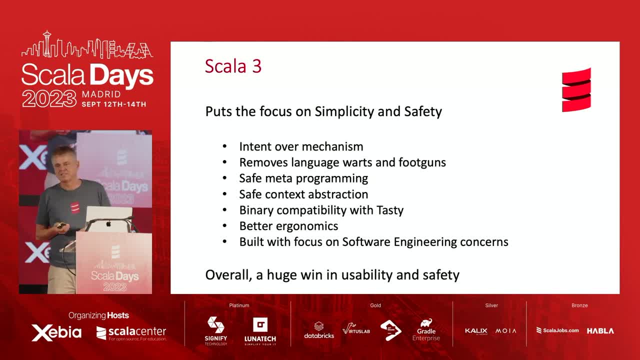 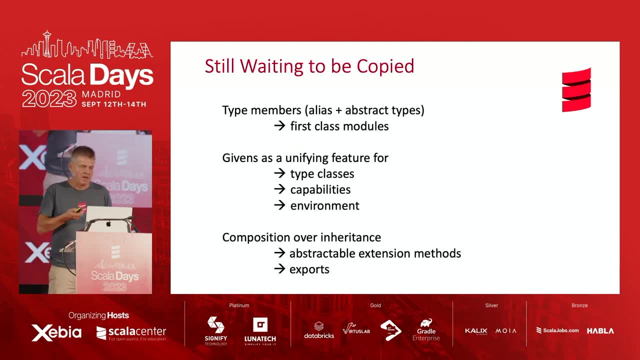 and safety. I'll talk about Scala 3 several times before, so I want to do that here. assume that we know all sort of what is this? but just in the abstract idea space, are that things in Scala 3 and also in Scala 2 that are still waiting to be copied by? 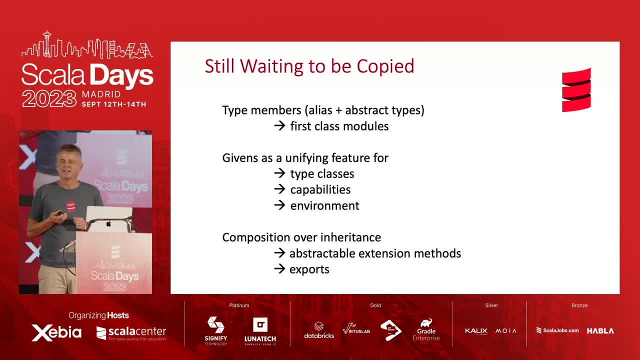 other languages. so what would I hope to see? that other languages would pick up, and a number of things, of course, from small to large, but three large ones that I think are really sort of important in Scala are those three. The first is type members, so that means alias types and abstract types as members of classes and traits, which gives us 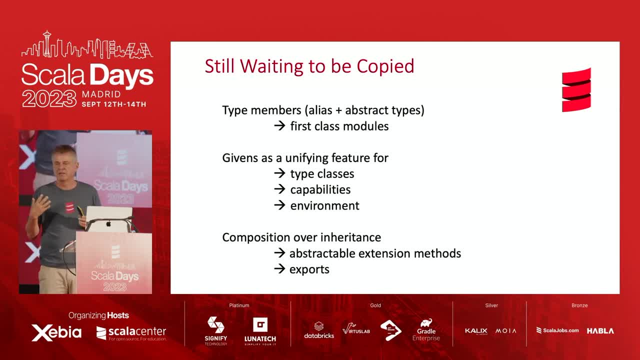 essentially the fabric for first class modules. So it means that's the reason why Scala has a really good module story, a really good story to put things together, and other languages haven't copied that much so far. The other one was the concept of Givens as a unifying feature of type. 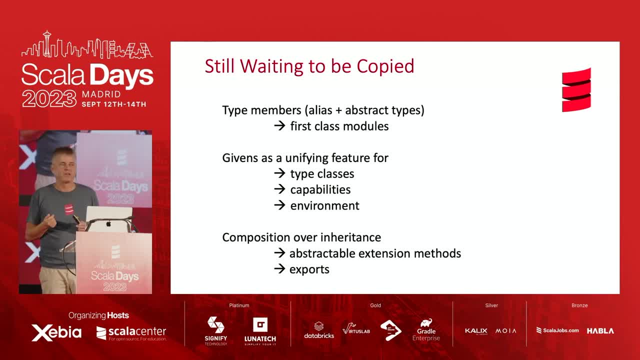 classes, capabilities and environment parsing. that's also something that I believe is something that's unique to Scala. Some languages are looking at it. for instance, OCaml is looking at so-called modular implicits, which are quite close to what we did there, but it's still something I think. Kotlin has contributed a lot to. But for some of the languages you timer then somehow gets epis��, message or something of the kind tofire you some sort of flavor aliases and you can't represent too much. you can just get it to your class And then, if you're like 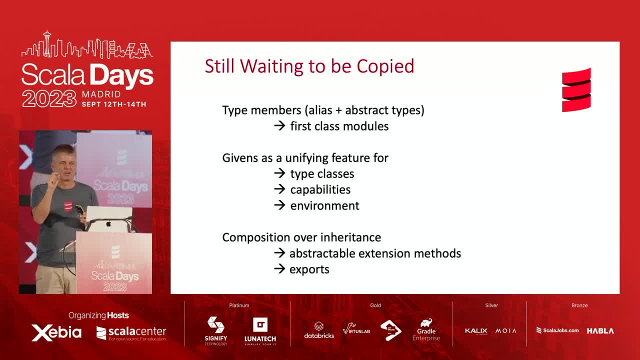 what about the Gr? waited for half an hour, see, and when I ask my test, nothing happened. Niklas says, if you need it, for half an hour with my test, and then the test is: oh, I can't keep. it has context receivers, which is sort of a very, very special case of a very, very particular 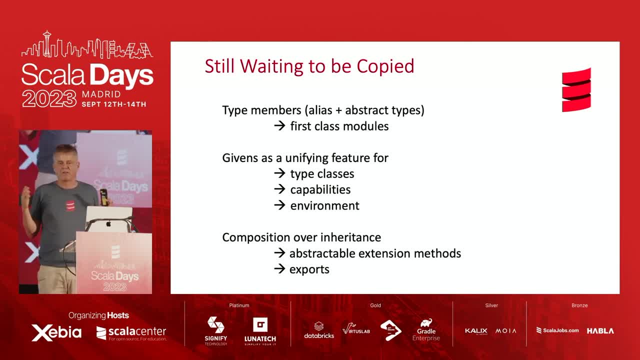 use case of this. But to look at it in its generality, it hasn't happened yet and I think is worth happening, because this is really sort of an important set of abstractions that one should learn from the roots, from the principles, from first principles and not 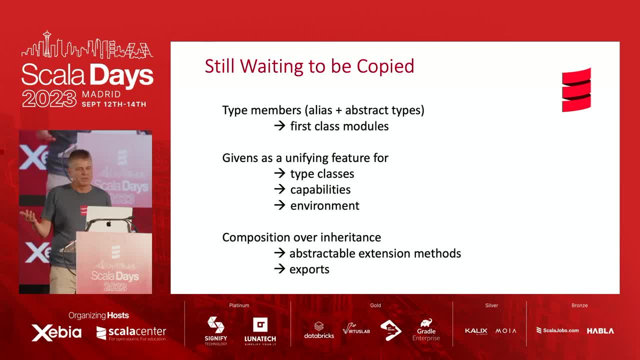 from some specific corner cases. And I think the third one would be to say: well, object-oriented languages, of course, have always been based with inheritance and we knew for a long time that that was not an unqualified good, that in many cases we want to prefer composition. 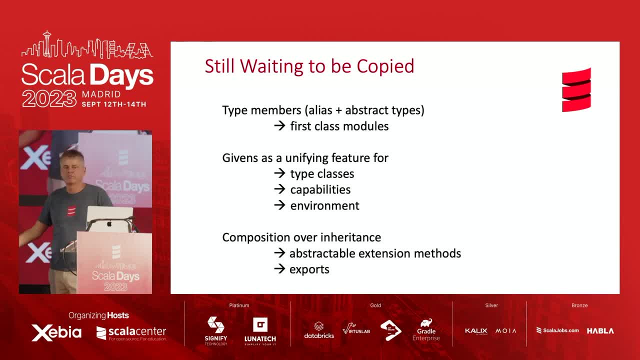 over inheritance, But that's easier said than done, because so far languages have made it very hard to use compositions. You had to write all these forwarders, a huge amount of boilerplate, to get this, This composition, and with both abstractable extension methods and export, Scala has now 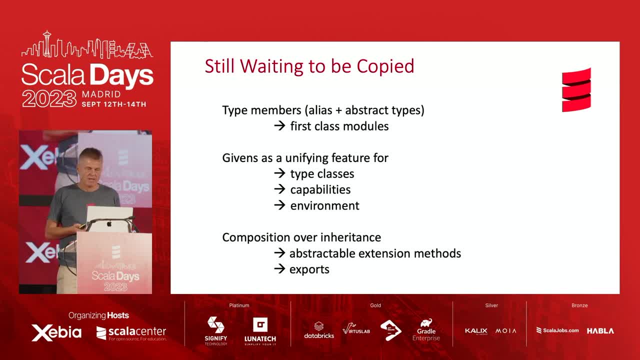 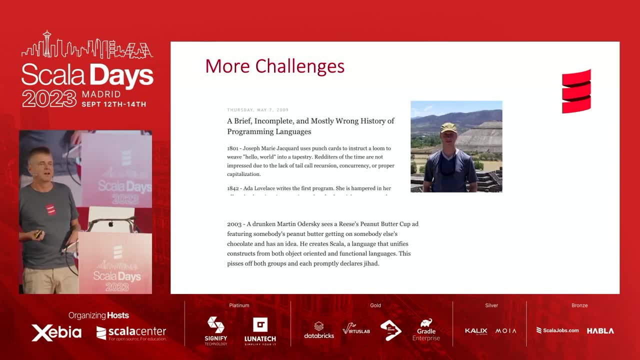 much better tools to achieve these things. Okay, so that was sort of the feature catalogs, But challenges are not just language features. There are other challenges as well, and they have to do essentially with the community, with the people applying the language. And so one challenge already came up in a very 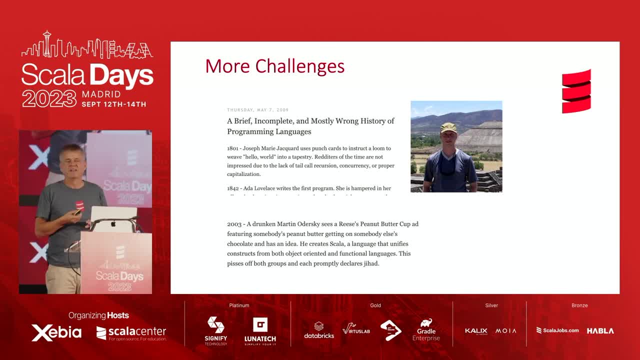 prescient blog post. It was 2012.. It was 2009, when nobody would suspect any of these things. There was this very funny story: a brief, incomplete and mostly wrong history of programming languages- by James Eyrie, And it's hilarious. You should read it, You should look it up. There are really. 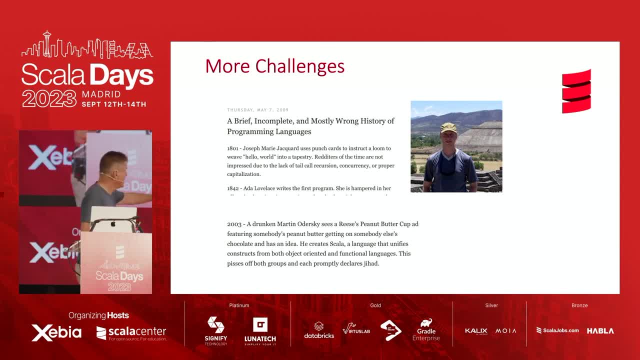 pearls about many other languages, But here's what he has to say about Scala. So he said, a drunken Martin Odetsky sees a Reese's peanut butter cup ad featuring somebody 's peanut butter getting on somebody else's chocolate and has an idea: He creates Scala. 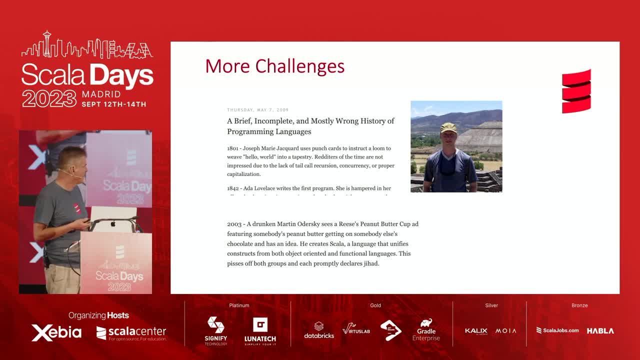 a language that unifies constructs from object-oriented and functional languages. This pisses off both groups and each promptly declares Jihad. Well, I think I was something to it, Even though at the time it's like, oh, this is a great joke, But yeah, good. So Jihad is a bit strong a word, But let's say we have. 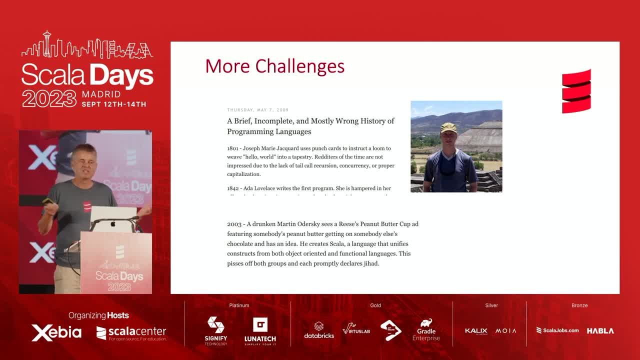 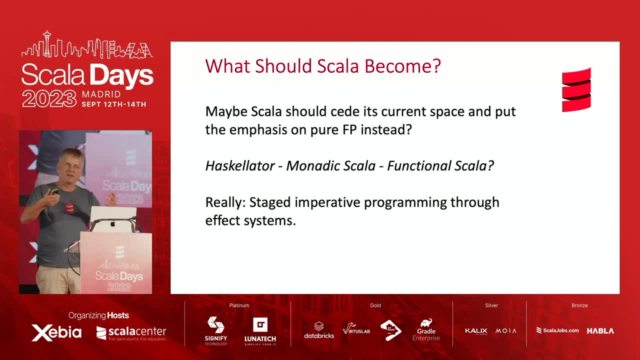 arguments. The Scala community definitely has this argument: Where should it go To? how functional should it become? So maybe one idea would be to say: well, if our languages go where Scala is, so Scala should move elsewhere. It should see this current space and put the 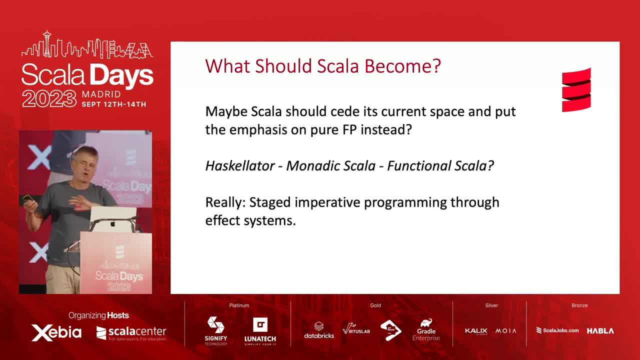 emphasis on even more functional programming instead Go all the way in for pure functional programming. And there have been various names for this: Functional Scala, Haskellator, Monadic Scala, several ideas to do that. So what this really means, because in the end, let's 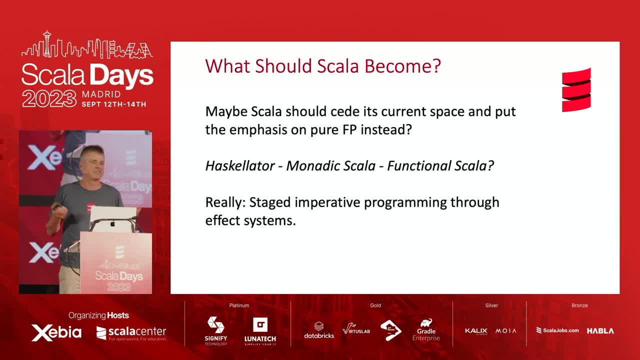 say, a Spark query is a functional program. right, It's functional. There's no side effect, There's no wires. But that's not what people mean when they say functional Scala. What they mean is really staged imperative programming. Your effects won't go away, but you will put. 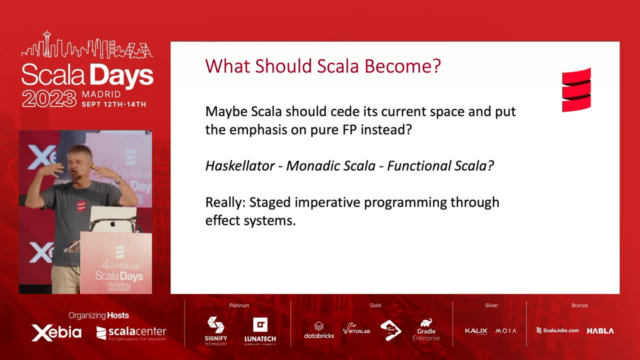 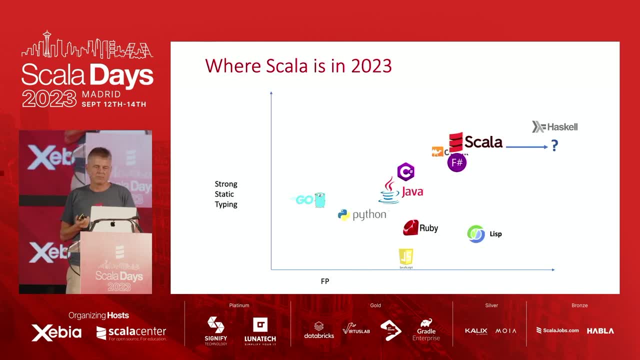 them in a monad and you will have a purely functional program that constructs this monad And then you hand it off to an effect system Runs your effect. So the idea there was to say: well, let's essentially go to the right. 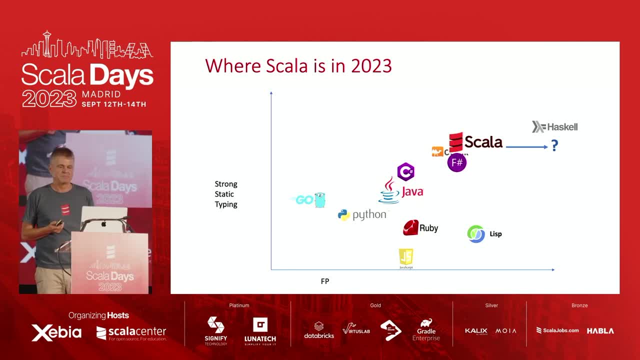 Let's move Scala all the way to Haskell And then maybe that way lies salvation. Personally, I don't think this is true. I don't think this is the way Scala should go. So just to give you probably know that, but just to state it on stage, I don't think it should do that. 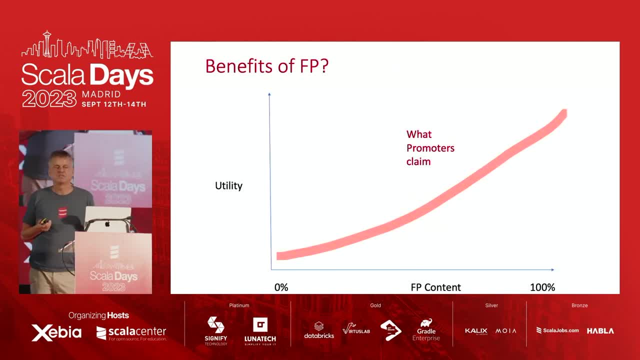 So, and personally I also think that the benefits of functional programming are not, let's say, it really depends very much on where you stand. So what promoters claim is: the more functional programming content your program has, the better. It goes even up when you go fully pure, 100%. That's like the best of all possible worlds. What 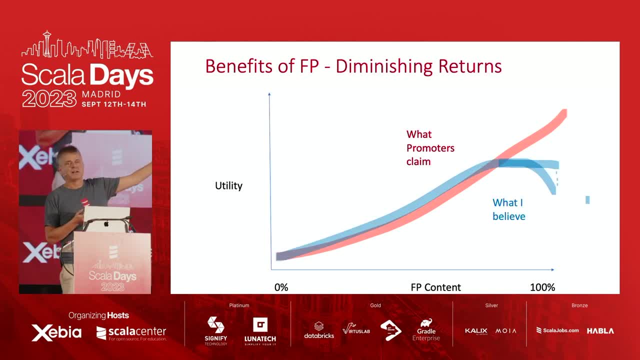 I think instead is that it goes up until you're about 90%. Definitely you want to be as functional as possible And afterwards the question is: it depends. For some programs it's worth to go to the 100% And for other programs it isn't. For other programs actually using, 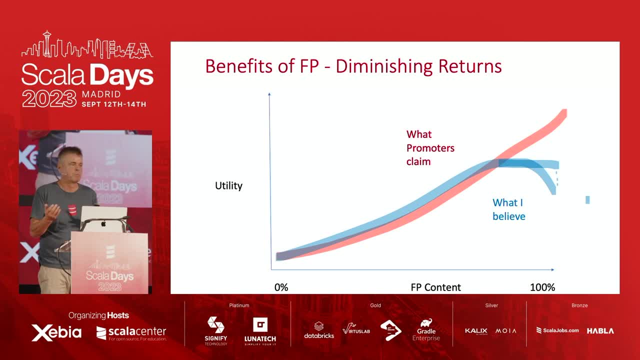 or renouncing on using state is counterproductive. You would be better off using a modest amount of state, And also that's why, very, very intentional, Scala is at the tip of the blue curve and to say: that's essentially where we want to be. 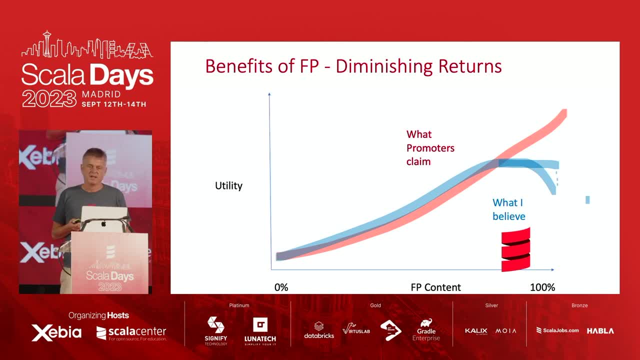 And that's what we optimize the language for. So, yeah, okay, I stated that like this, and I realize it's a contentious question, so I should back this up. So I want to back this up with some examples which come from code that I have either written myself or 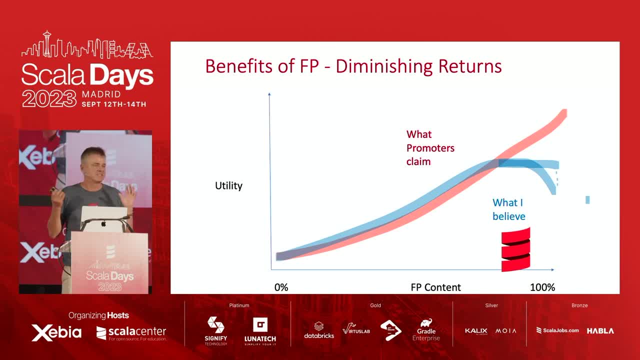 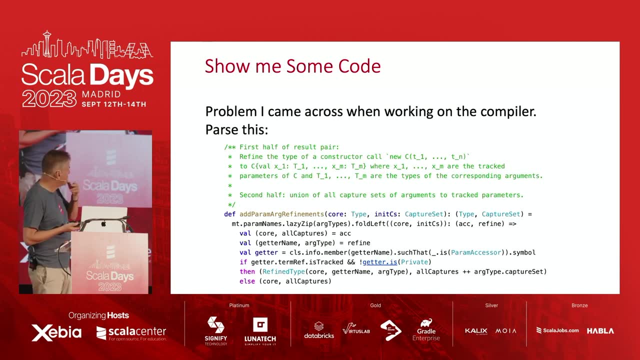 seen myself and that's code in the compiler. So these are real use cases. They're not made up. So one thing, that's code I had written myself. And then I realized I wrote that code six months ago And I said: well, this seems to. 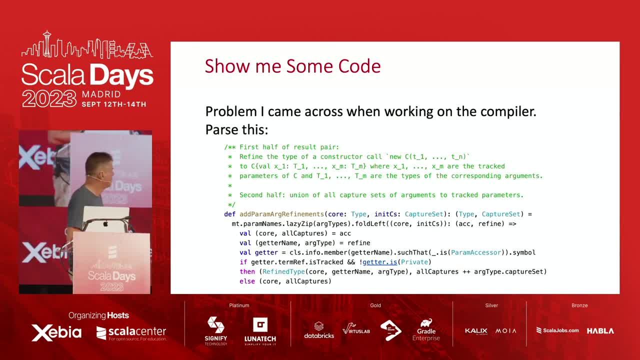 be a bit harder to understand than other code. So well, yeah, so there's a big document, So I didn't skimp on the documents. And the document is actually correct. It tells you what it does. But even when you read it, it's a bit hard to essentially do all these unpackings. 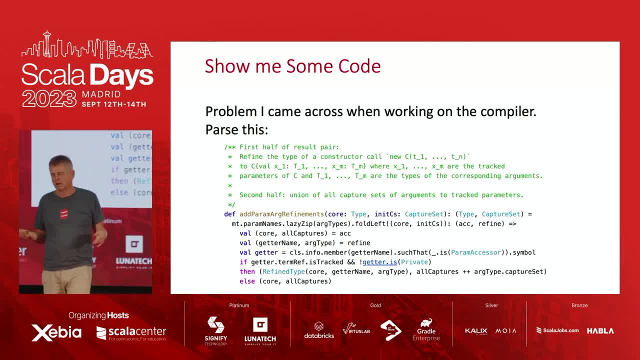 and things like that of this fold left. So, yeah, I looked at it And after about five minutes or ten minutes maybe, I said yeah, yeah, okay, yeah, all good, I understood it. now I said, yeah, but maybe one shouldn't have to spend even five or ten minutes to. 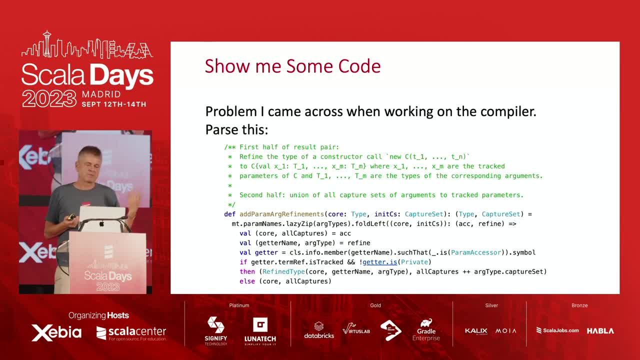 understand code. Code should be obvious, right? So then I said, well, a challenge, Martin, make this code better, How can you make it better? And I said, well, I used the fold left. Another thing to do these sort of things is with using recursion. It could be a tail. 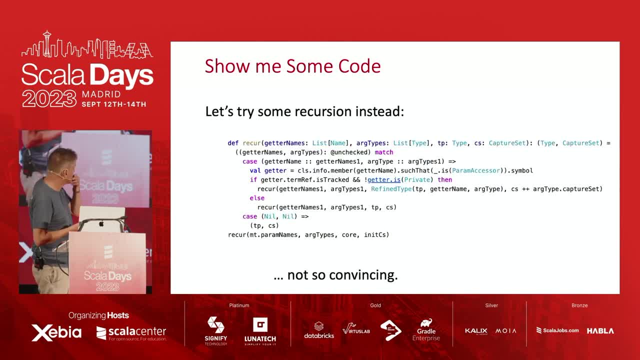 recursive function. Let's try that. So I tried that What I came up with? well, it got maybe clearer if you read through it. There were no hurdles to sort of understand that. But it also got a bit longer. So overall I said no, that's. 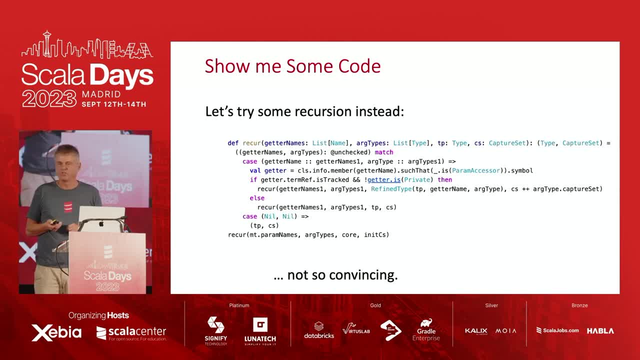 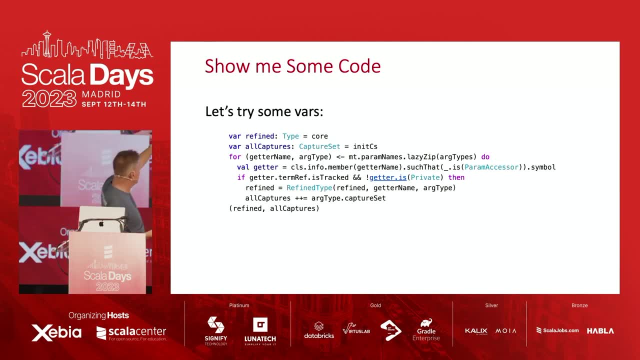 not so convincing. I said, well, now let's read for the poison cabinet and do some vars. And then suddenly it actually did get better. So now this code I actually am not ashamed to read to you. So we have two quantities refined and all captures, a type and a capture. 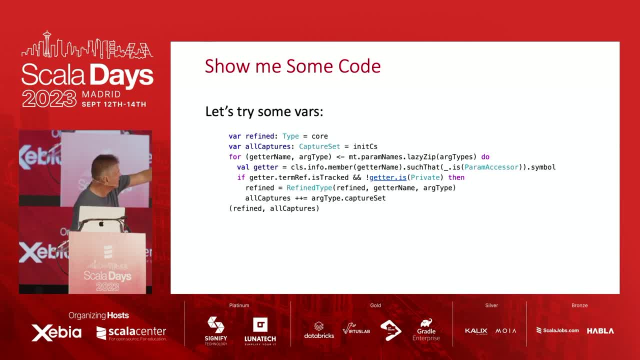 set And what we do is we go through parameter names and argument types, We zip them together And that's a getter name and archetype. Then from the getter name we produce a getter And we say, if this condition is true, then we update both refined and all captures to. 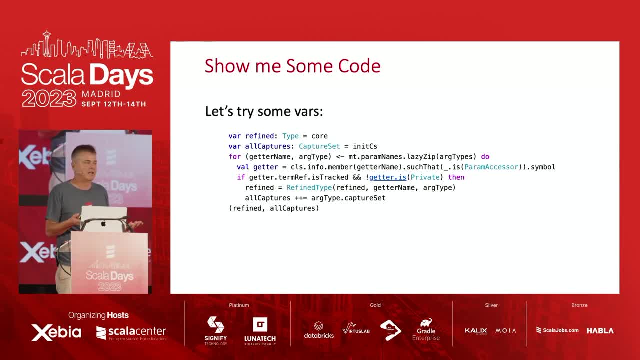 the next value. So this is all very, very obvious and clear. So I would say, well, in this concept, that's actually the clearest solution. You could say, yeah, but Martin, isn't that bad, You're using vars. I thought you wanted to be functional. So is that code still purely? 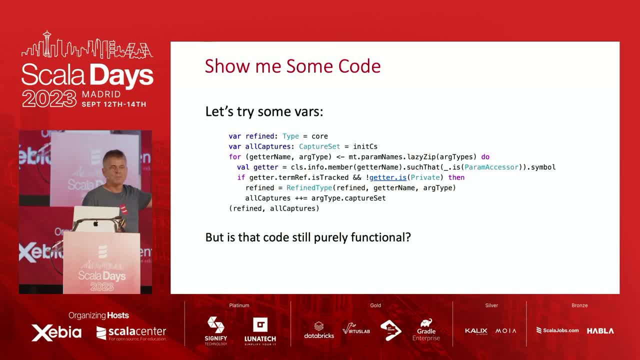 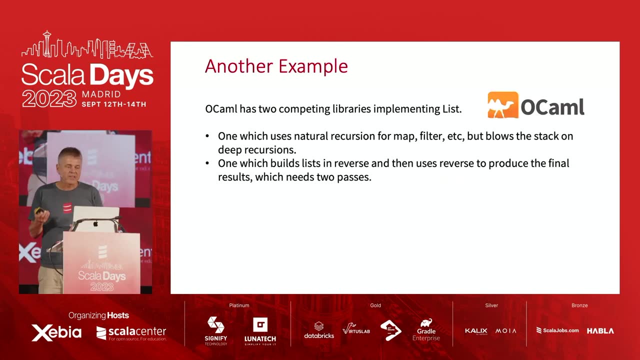 functional. Well, the point is, from the outside it's absolutely purely functional. It's exactly the same function that I wrote before. I used two local vars internally to make the code clearer, But from the outside this is still a pure function in the mathematical sense. 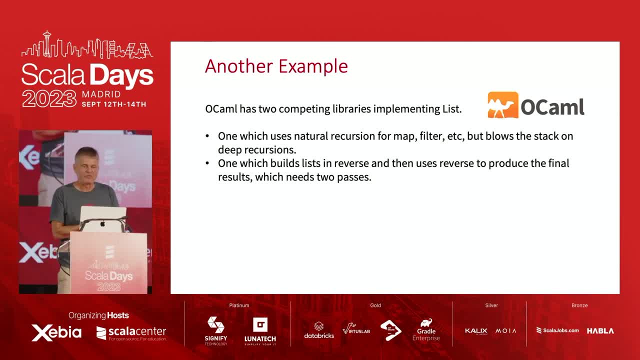 Another example, and there I am looking first at another language. One curious thing about OCaml was that it has for a long time had, and still has, two competing libraries that implement lists. The most basic data type of them all has actually two competing implementations. 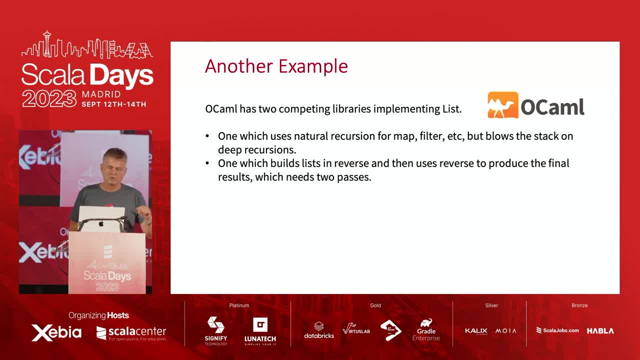 one by Jane Street and the other by INRIA. One uses natural recursion for map filter, but that blows the stack if the list gets too large, And the other builds lists in reverse and then uses a reverse to get two reverses to produce the final list. So that's a very 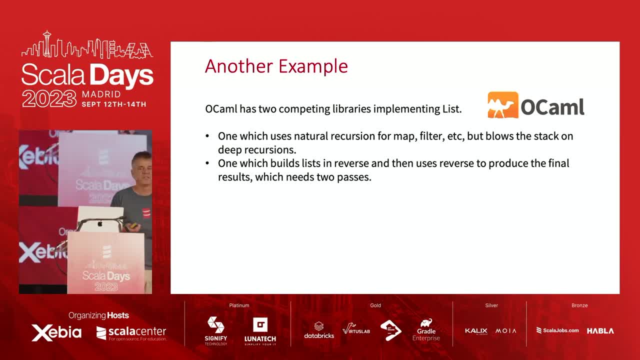 tricky thing to do. So what's the problem? Well, like I'm sure you've heard of this before- the parameter is a list, So that is slower, It needs two parsers, but it is stack-safe, so you don't blow the stack with long lists. So that's an awkward trade off, right Are? 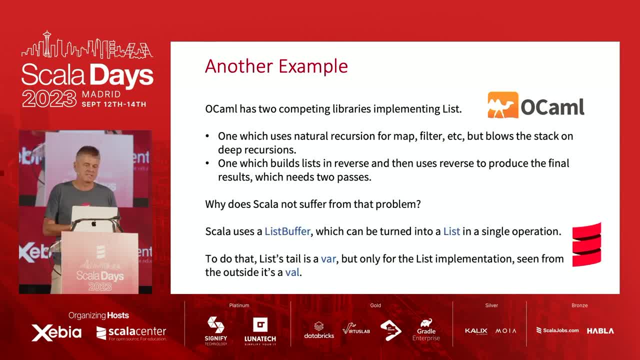 you stack-safe or are you fastest and most natural? So what does Scala do in that case? It doesn't have that problem at all. What Scala does? it uses a list buffer, and the list buffer can be- once it's completed, it's an imperative structure, of course- can be. 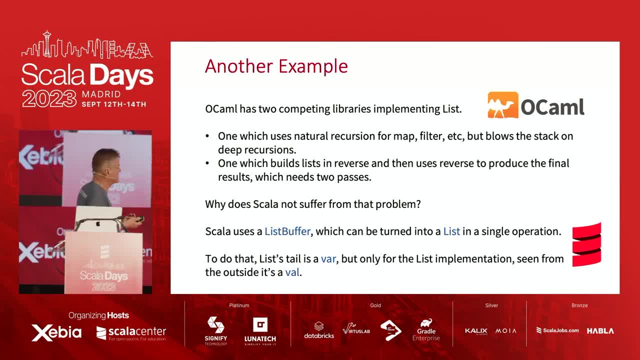 a single operation. And how does it do that? The internal workings, actually, if you look at the source code of list, then you will actually find out that the tail of a list is a var, What It's a var, I mean. who could change the tail of a list when it's actually a var? only for the Scala. 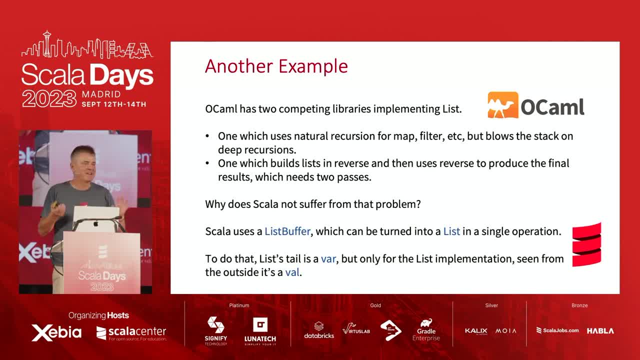 library. It's not available to you, So it's only when you maintain the Scala library, then it's a var and then we need it to be a var in order to be able to implement this very fast single operation to turn a list. 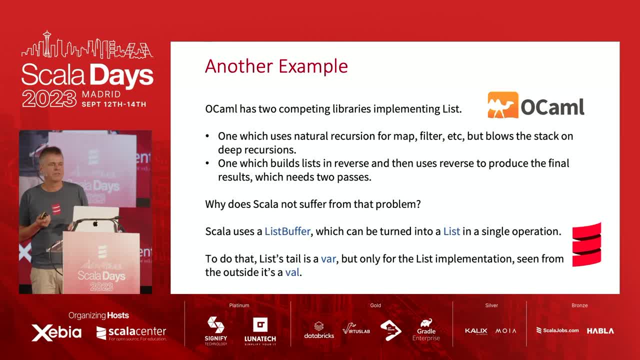 buffer into a list. You could also say, yeah, but that's dirty right. Yes, but we have essentially the best of all possible worlds. We have the fastest implementation of lists and it is stack safe. So it's definitely worth putting a bit of essentially tricks in there. 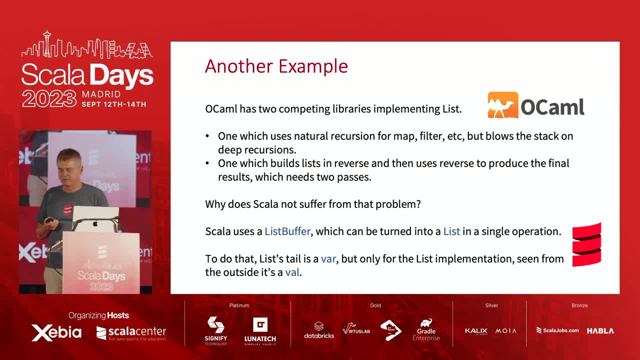 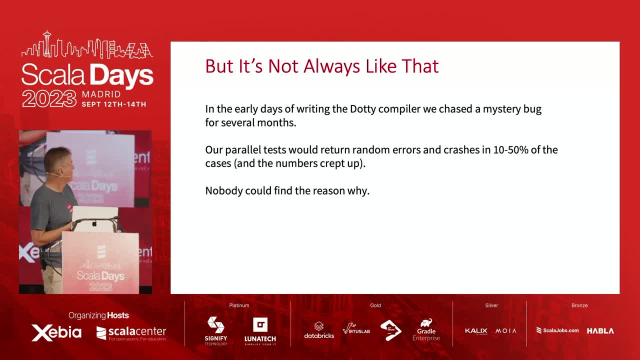 Okay. so I've given you two shiny examples where vars actually really help, but I should admit It's not always like that. So another thing, also from experience, is in the early days of writing the DOTI, the Scala 3 compiler, we chased a mystery bug for several months and it got worse and worse. 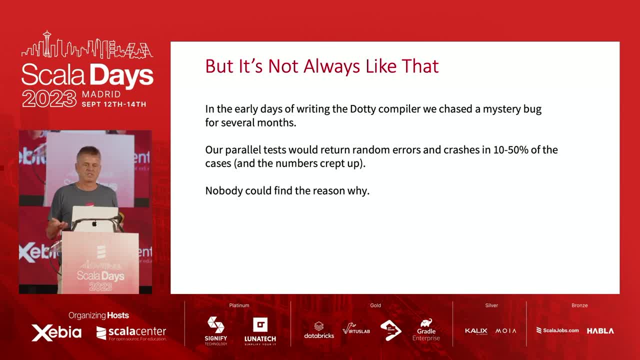 So our parallel tests would return random errors and crashes in 10% to 15% of the cases. when we ran the tests and the numbers crept up, the more tests we added And nobody could find the reason why. We looked everywhere. 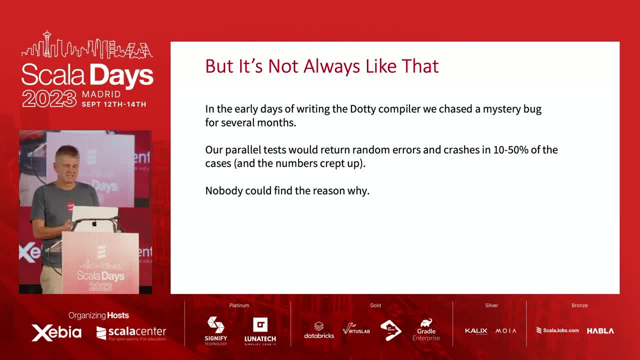 For months we looked everywhere and we couldn't find why these tests were crashing. So randomly crashing tests means it could be a data race, right, But where? Where was the data race? And we couldn't find it. So in the end, I actually wrote an analyzer that would reject any globally accessible. 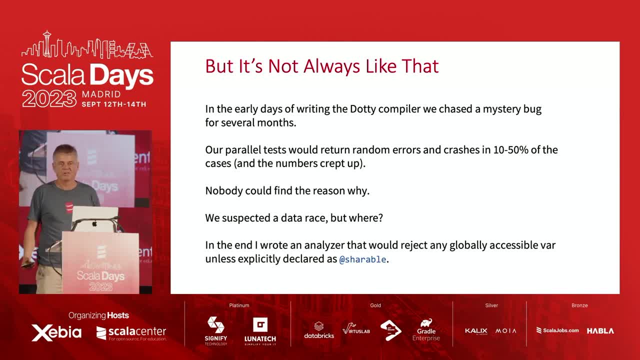 var, unless explicitly declared as shareable. So just to say, anywhere in the code base, let's write a tool that could bring up all these possibilities and that actually found it. So what we found? we found a problem in a file with the index. 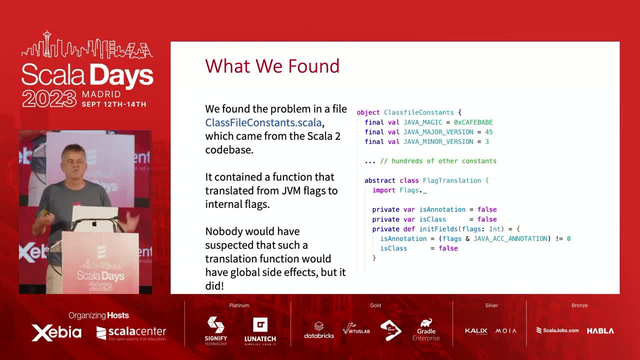 Innocuous name class file, constants, dot, Scala. So who would suspect anything wrong in that? And that, furthermore, came from the Scala code base. That's why we didn't look at it very closely, because we thought, well, that's probably. 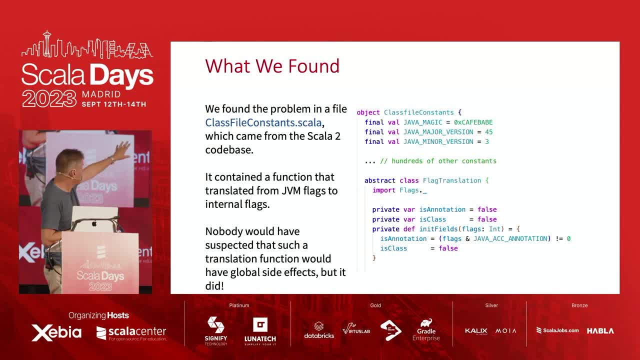 OK, It worked for 10 years in Scala 2. And that contained a function that translated from JVM flags to the internal Scala flags. You see flag translation. why would that use state, global state? Nobody would have suspected that That sort of translation function would have global side effects. 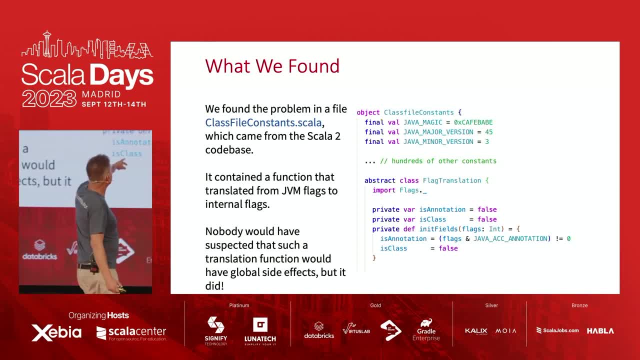 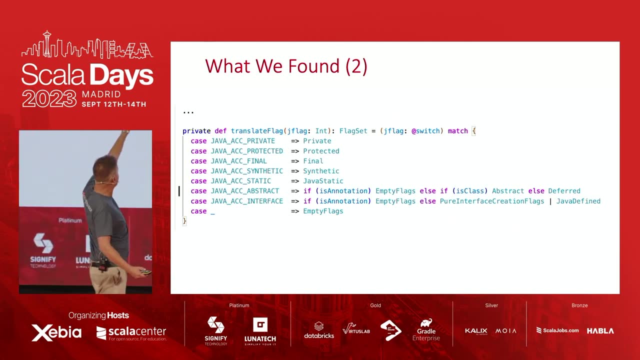 But it did And you see that on the right here. So there's actually a class flag translation And it has two fields: is annotation and is class And those are set by the init fields method And they are queried by the translate flag method. 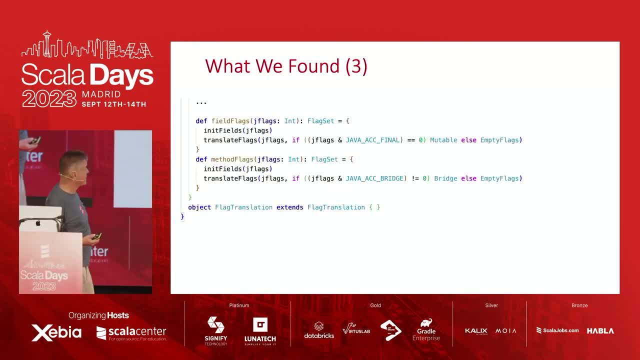 And then there's the field flags and method flags method, which is the external API, that both do an init fields and then are followed by a translate flags. OK, You say good, Still no problem. These side effects, maybe they are stashed away. 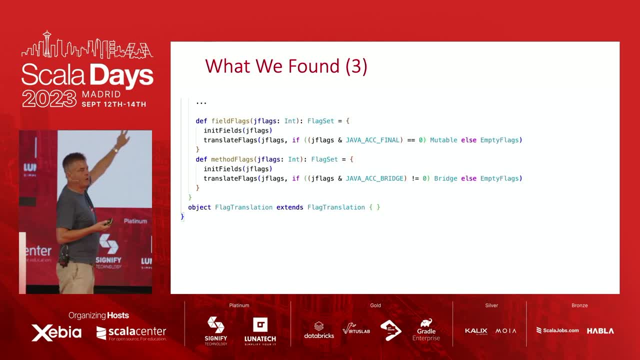 But the reason is, the reality was no. There was a global object, flag translation that did it all. that extended this abstract class. So in the end you had two global variables is abstract and the other one. And what happened then is that, as we ran, 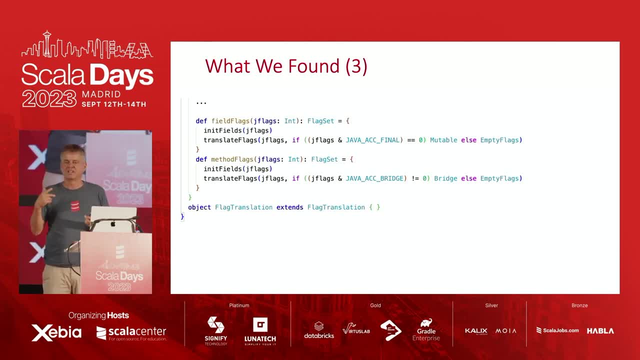 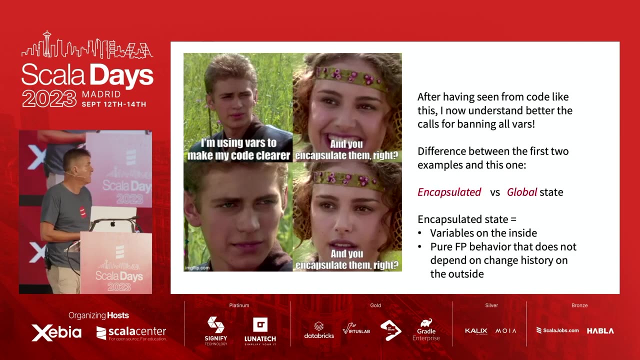 As we ran more and more tests in parallel. these things would essentially have race conditions: that several init flags would happen at the same time before the flags were queried, And so the flags would randomly get across each other. After having seen code like this, I now understand better why one calls for banning all virus. 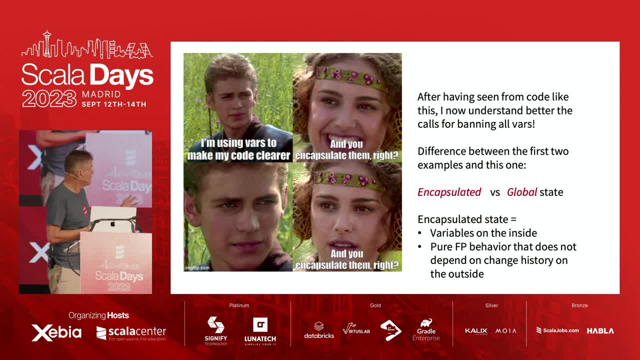 That definitely cost us a lot of time. So the difference between the first two examples and this one is that The first two examples I showed you encapsulated state. So we have state, We use state, But to the outside it's a purely functional interface. 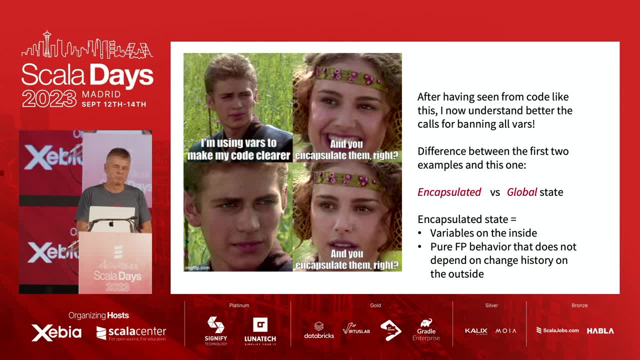 There's still purely functional lists. It was still a purely functional method, But here we had- by accident probably, introduced global state, a state that essentially was visible to the program globally. So encapsulated state is sort of the nice part of state where we have variables on the 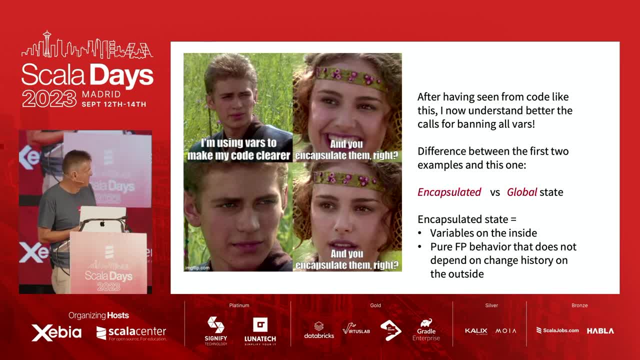 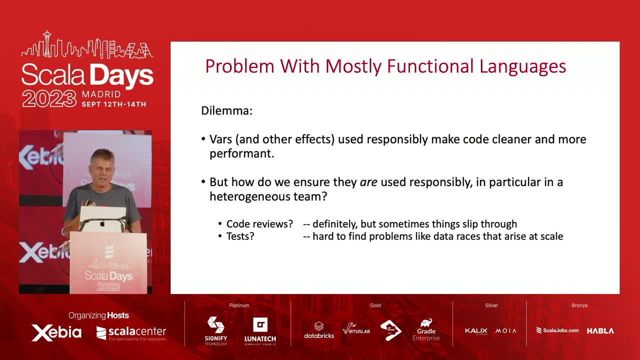 inside and pure functional, Functional behavior that does not depend on change history on the outside, Because they're the Okay. So one problem, going back to language design now, is to say: well, if we want to say we want to have a mostly functional language like Scala is where we say we have state. 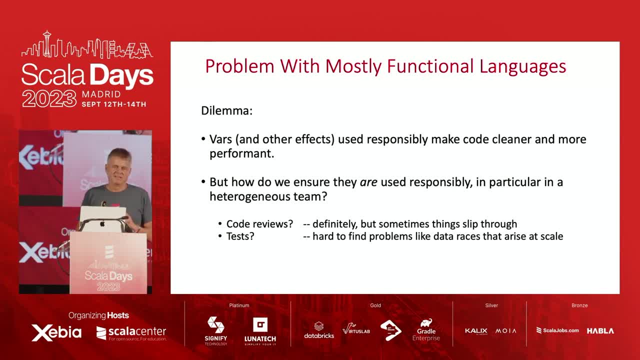 use it responsibly, then the question is: well, how do we make sure that these virus are used responsibly? Obviously, Sometimes they aren't, So we would like to use them to make code cleaner and more performant. But yeah, how do we make sure that everybody plays by the rules? 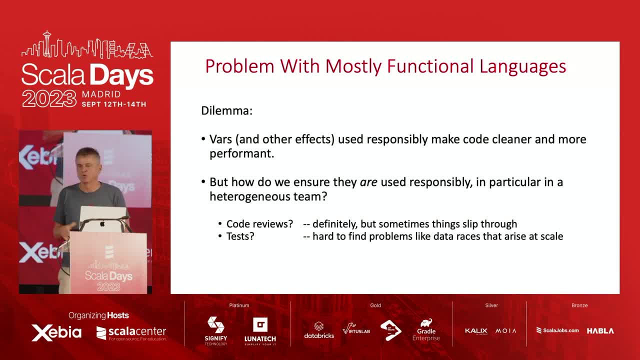 Code reviews definitely, But sometimes they slip through. Here it was because it came from a different code base where we didn't suspect it. Tests, yes, also, But in a case like this that essentially only was The problem, only was visible at scale. 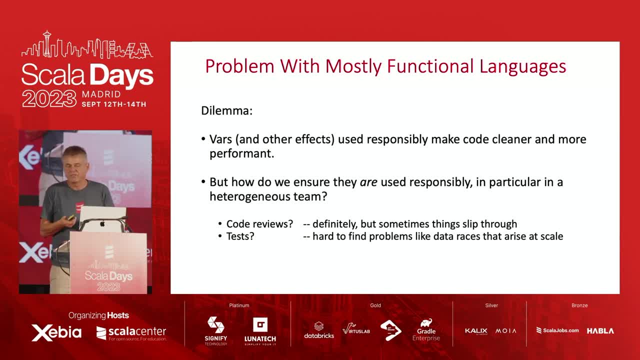 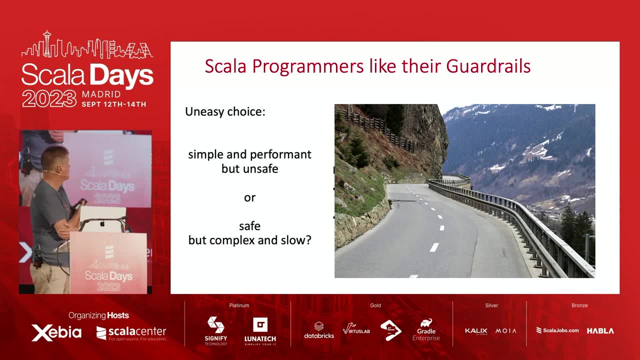 So when you had lots and lots of parallel, Lots of parallel tests running together, So it's very hard to write a unit test, for instance. So that means Scala has an uneasy choice: that we can be simple and performant, but in the 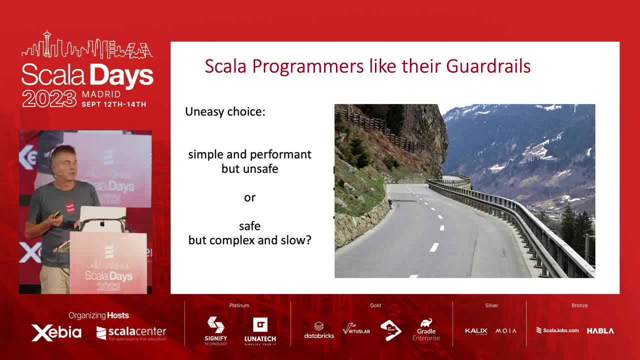 end unsafe. We have to accept a certain degree of unsafety, or we can be safe, but we have to accept certain trade-offs that will become more complex in places and maybe slower in places as well. And yeah, let's face it. 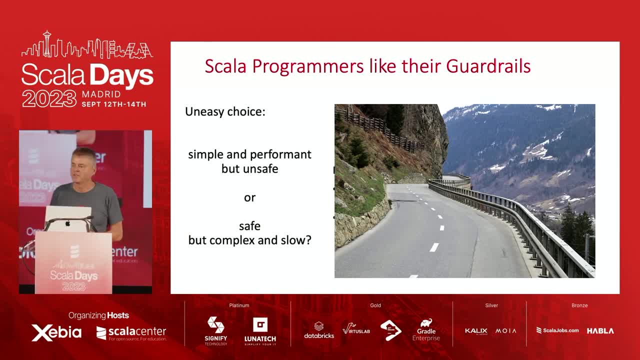 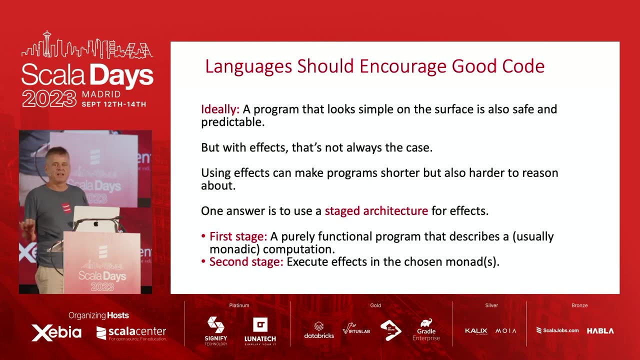 Scala programmers do like this. They like this. They're guardrails, And the fact that essentially we have these unprotected wires it makes some people uneasy. So languages, of course, should encourage good code. So ideally, my ideal would be that a program that looks simple on the surface is also safe. 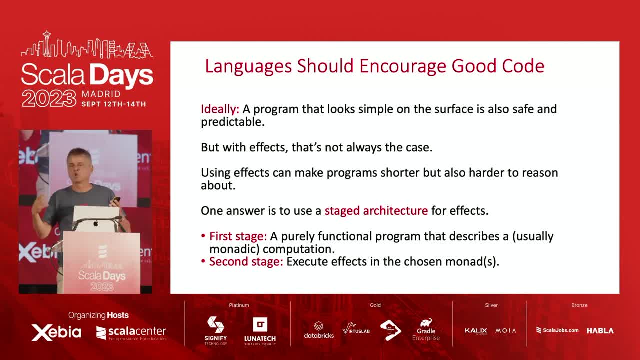 and predictable. So essentially, the notation should guide you towards the right decisions when you write your programs. That would be the ideal, But we've seen. We've seen that with effects that's actually not always the case. Using effects can certainly make your program shorter, but sometimes, if you use them wrongly, 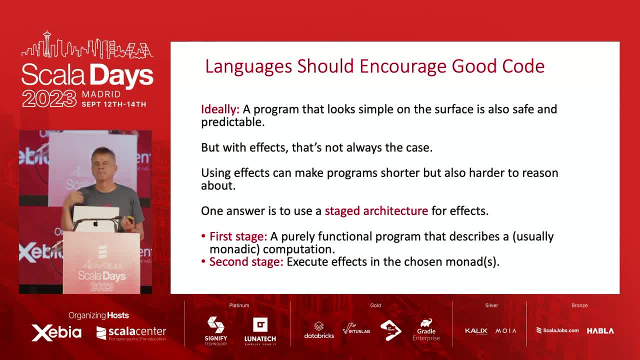 also harder to reason about. Now, if we would all reason about our code from day one, that wouldn't be a problem, because you would say, well, this is too hard to reason about, We don't. But let's face it, We don't do that. 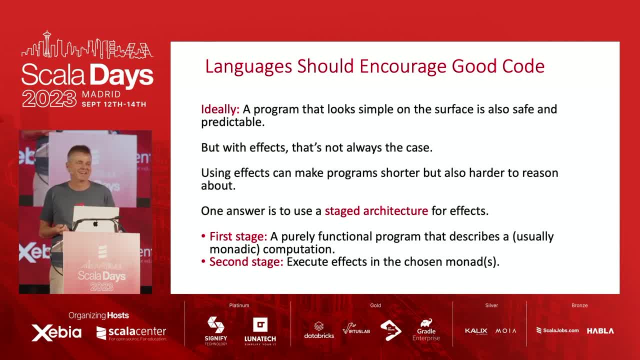 We just write our code and then things slip through, and then the next people who maintain our code, maybe they have to bear the consequences. So one answer to that would be to say: well, we use a staged architecture for effects. That's the answer of effect systems. 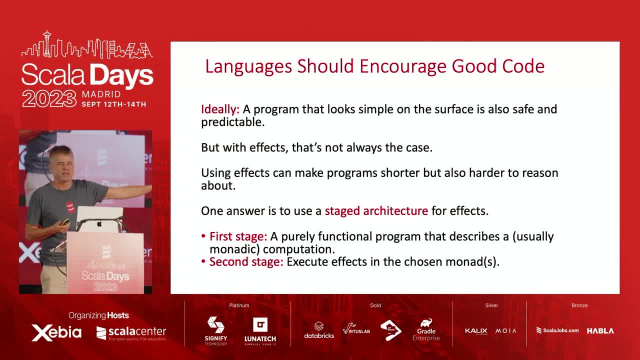 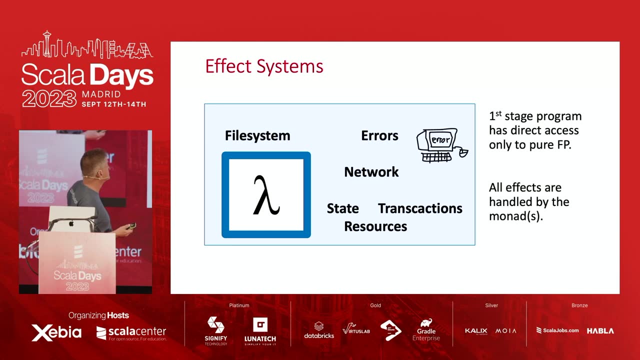 We have in the first stage a purely functional program, no effects allowed. that describes a usually monadic computation, and in the second stage we execute the effect in the chosen monad or monads. So what that means is a system architecture like this one here. 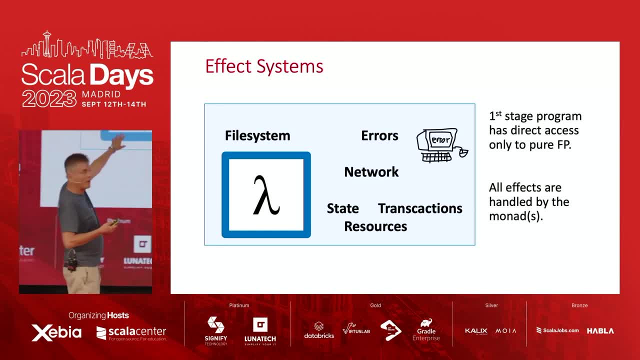 So where we have a purely functional program, the format gives us results And at this moment we see that the best outcome we're getting is an as-is approach, So we're kind of forgetful. functional program- that's a big lambda that you see here and it's in a very rigid box. 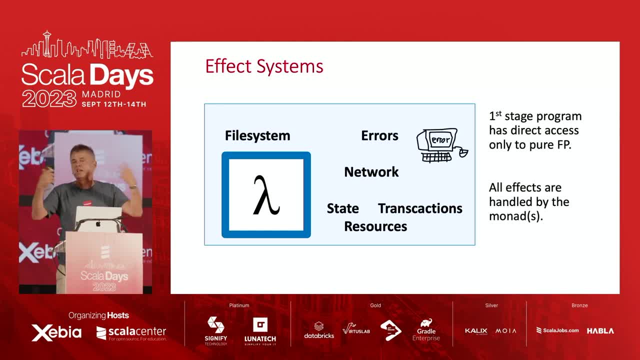 which says: well, that's essentially all you can do in your program. but what you can do is you can produce a value, a data structure or something like a data- in the end, a data structure that can express and affect full computation, and through that data structure. 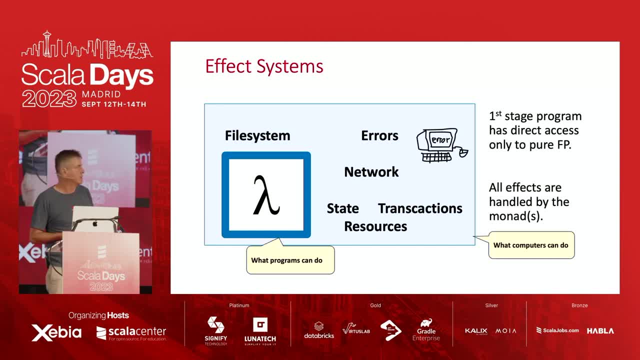 you reach out to all the things that computers can do. So the inner box is what programs can do purely functional. the outer box is what computers can do. all these things from handling errors, network state transactions, file system, other resources and so on. 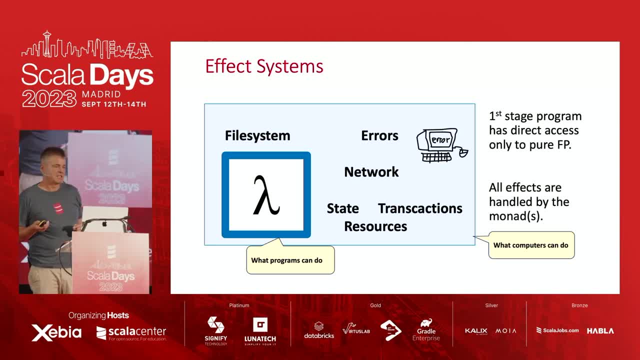 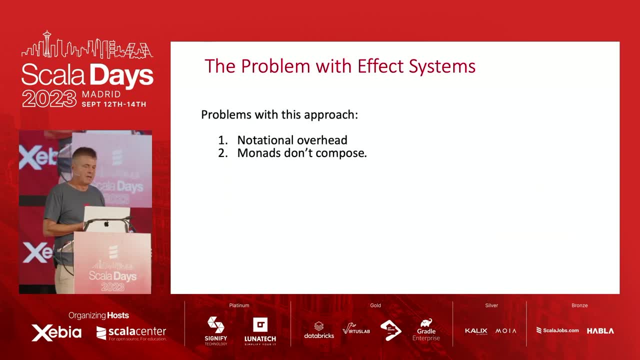 Okay, so this looks like has been a standard architecture for quite a few years and it looks quite reasonable, but there are also problems. The problem with this approach is: first, it leads to a fairly high notational overhead usually, and the second problem 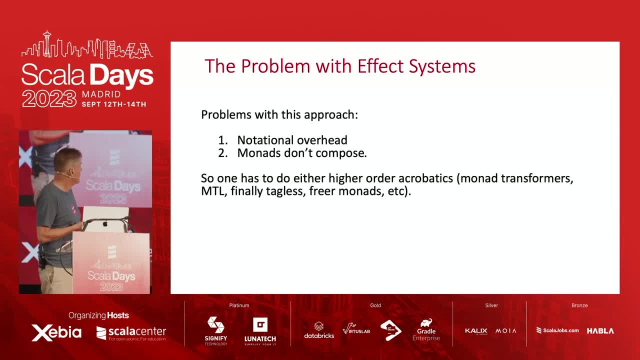 is that, unfortunately, monads don't compose, So one has to. essentially, instead of putting monads together, one has to put something else together, like monad transformers, or one uses finally, tagless, freer monads. Over the years there has been a cottage industry. 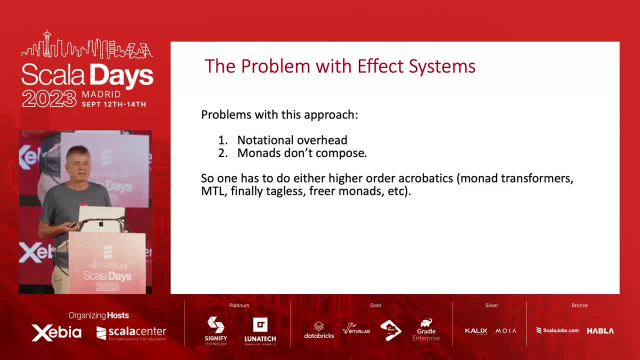 of approaches to essentially solve this problem, but I think it's also fair to say that none of these approaches ultimately has won everything over. Or the alternative is put everything into a single supermonad, But that can lead to over-provisioning. Do I really need three type parameters for everything? 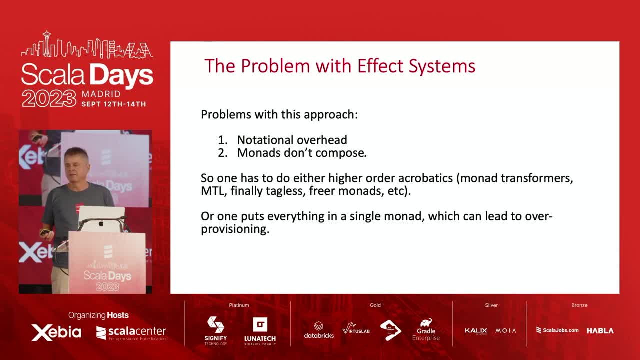 I do. Well, there are some situations where I need them, but by going with a supermonad like Zio I say, well, that's essentially now what all my programs will look like. So I would say the industry experience with this has been mixed positive in some places. quite 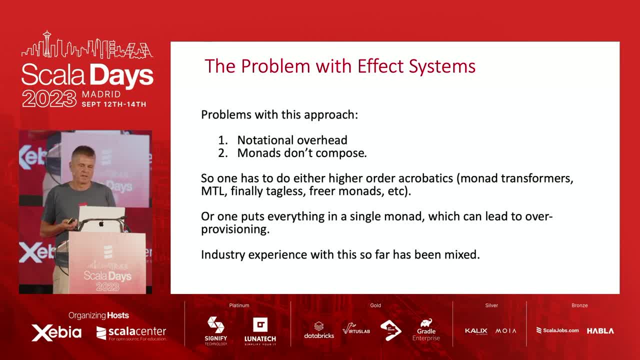 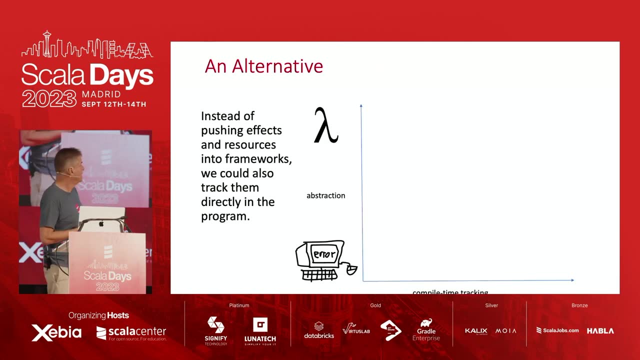 challenging in other places. Yeah, So there has been recently an alternative, a kind of pioneering- in academics by algebraic effects and in practice by languages like Rust and others, where the idea is that instead of pushing effects and resources in frameworks, we want to upgrade our type systems so that we can track them directly in the program. 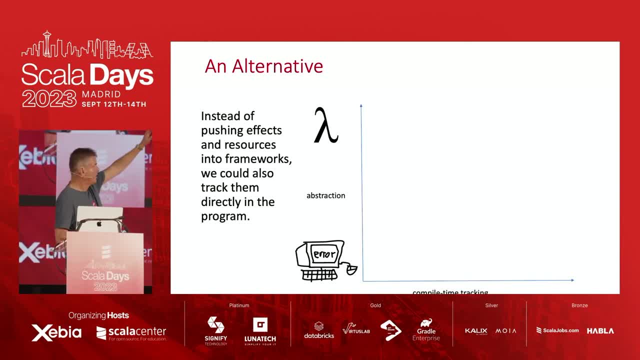 So here I have sort of this thing, two axes. The vertical axis is abstraction from the gnarly low-level world of computers to the digital world of computers, And the vertical axis is abstraction from the gnarly low-level world of computers to the digital world of. 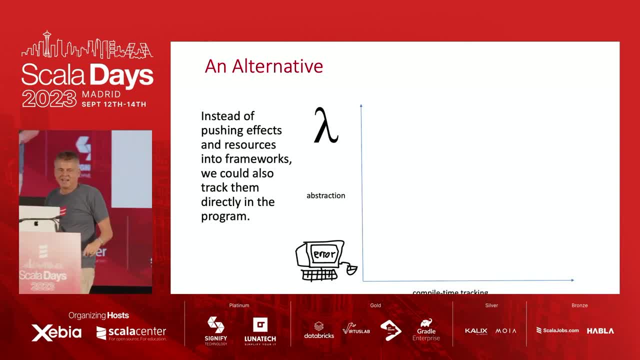 computers. And the vertical axis is abstraction from the gnarly low-level world of computers, A very lofty high world of lambda calculus programs in computer science and operation agencies. and the right axis is compile time tracking. to what degree does my language and type checker allow to track what kind of effects I use and what kind of? 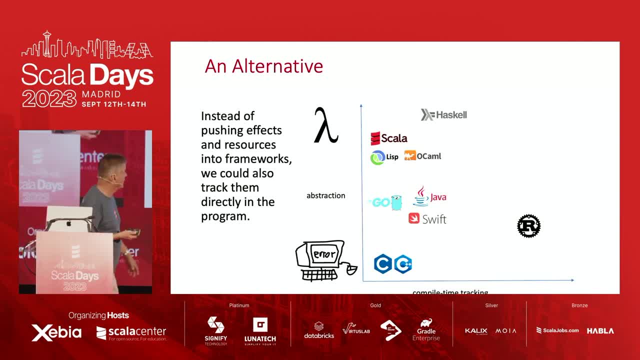 resources I use. And if we look at languages here, well, there are obviously languages at different abstraction levels. C, C++ is very imperative. Scala and Haskell are very functional. They're high up there In compile time, tracking almost all languages so far. 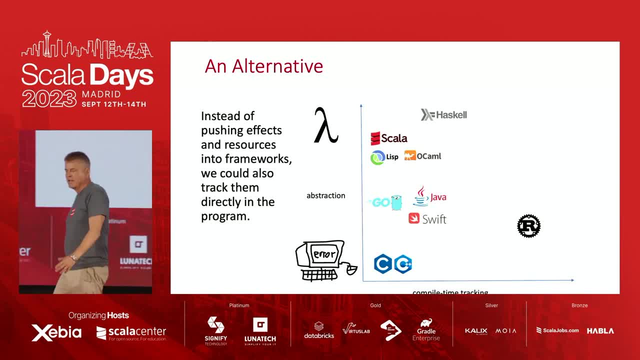 are pretty much to the left side of this quadrant, except for Rust, which is a relatively low level language. That means it's quite imperative everything you express, but it has a very precise tracking of effects at compile time with the borrow checker. 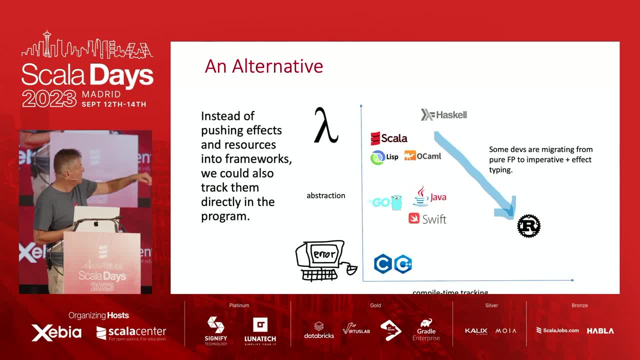 And what's interesting is that quite a few people are migrating for pure functional programming to imperative plus effect typing, and they don't find it so terrible. The feeling you get is: well, as long as the compiler has my back, maybe effects aren't. 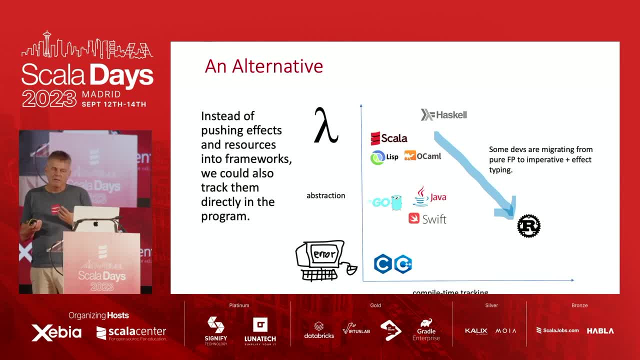 so bad. But what I think is it's kind of a pity that in doing that, you have to lower the level of abstraction, You have to become more inflexible, You have to worry about resources all the time, Everything has to have limited lifetimes, and so on. 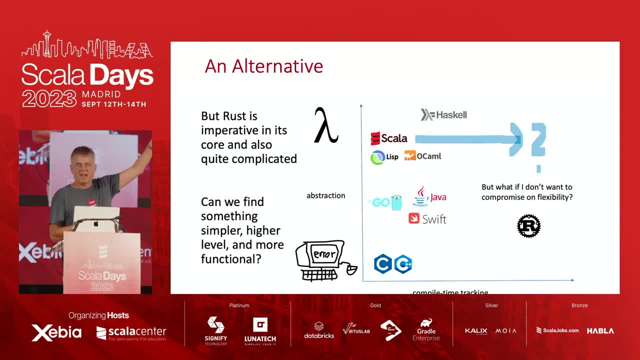 So I wonder: why can't we do the same thing But stay on the nice and functional level of abstraction here on the upper right angle? And that's what we are trying to achieve with the new project that we have started this year called CAPRISE. 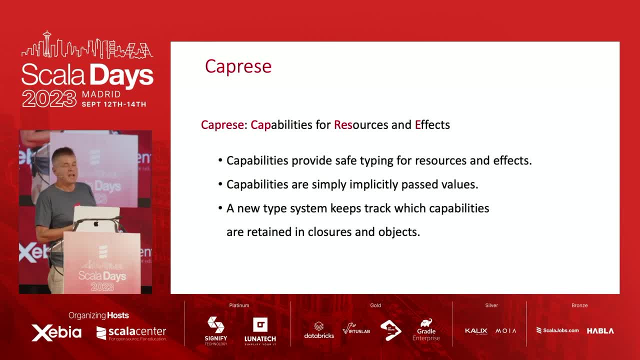 So CAPRISE is an acronym for Capabilities for Resources and Effects. So the idea of CAPRISE is that we want to express capabilities that provide safe typing for both resources and effects. The idea is to have an effect. you need a capability to have the effect and we track. 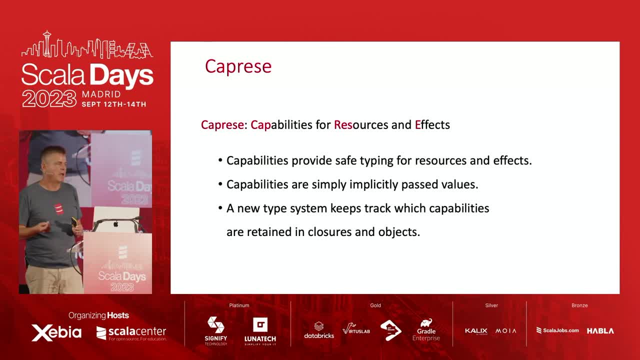 that, What is a capability? Well, a capability is simply a value that I give you, that I pass off, an unforgeable value. And because of ergonomics, I want to make this passing of capabilities implicit, That is, if I say, if the caller has a capability and the callee needs it, well then I don't. 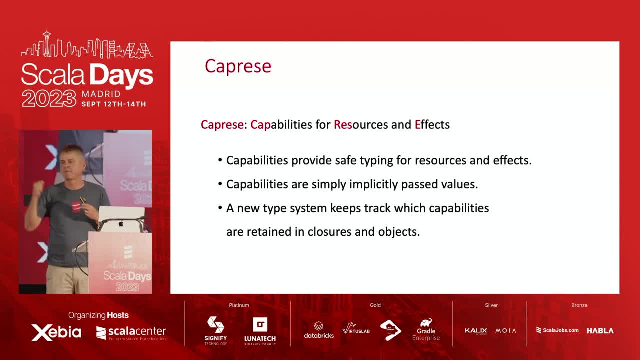 need to go through procedure and ceremony to pass the capability to the caller. It's simple. It simply gets passed as an implicit parameter. So SCADA's implicit parameters really fit that like a glove to a hand. They're a very nice concept for that. 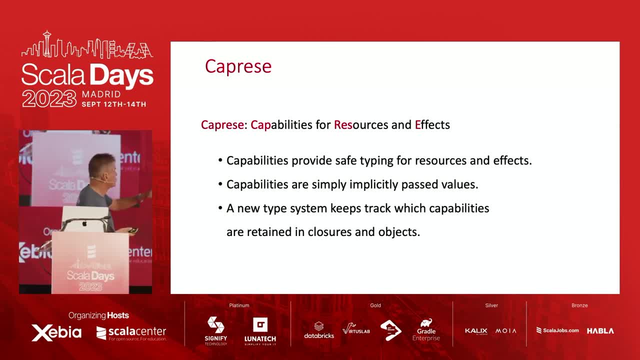 But there's one thing that we also have to do is we need to track, keep track which capabilities are retained, enclosures and objects. If I have an object, I need to know what effects can it do, what capabilities does it have inherently, without getting something else from the outside in a parameter. 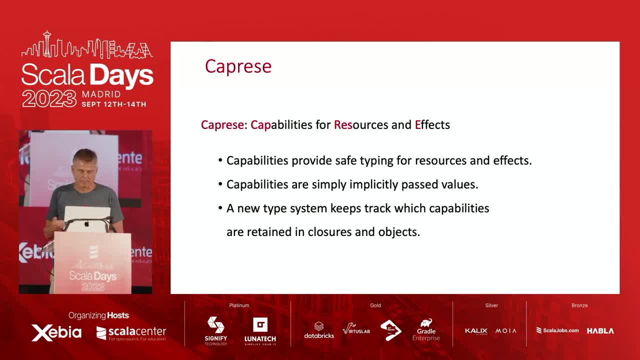 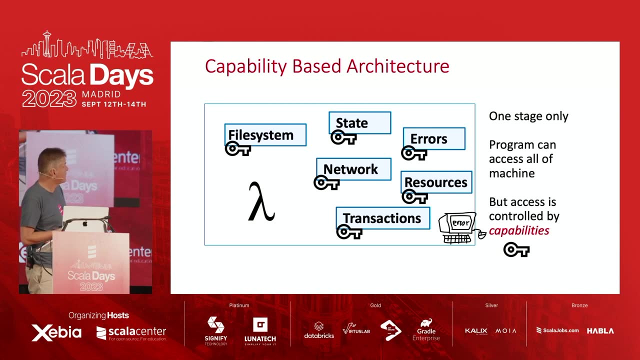 And that has been missing so far, And essentially, with Caprizi, we have developed the type, systematic foundations for that, And we have developed the first implementation for that, And now we have to push it further. So what that can lead to is a new kind of architecture, which is known as capability. 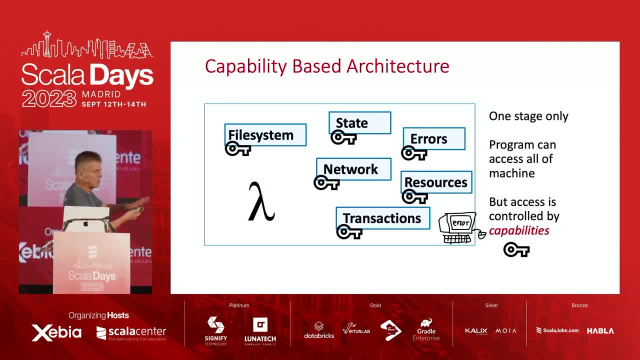 stage based architecture, which is not staged as the previous effect systems. It's one stage only Your program can do, has access to everything The computer can do, But they are all all require a key. So the key is essentially the capability. 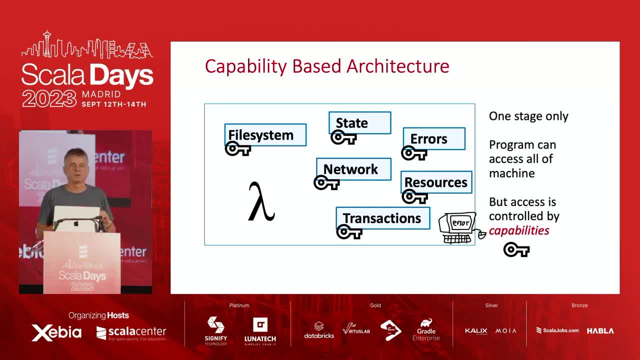 If you don't have the capability to essentially access a network, you can't access the network. Of course that's a very old idea in security and operating systems and so on. The novelty here is we have now. we have that now in a programming language and a type system. 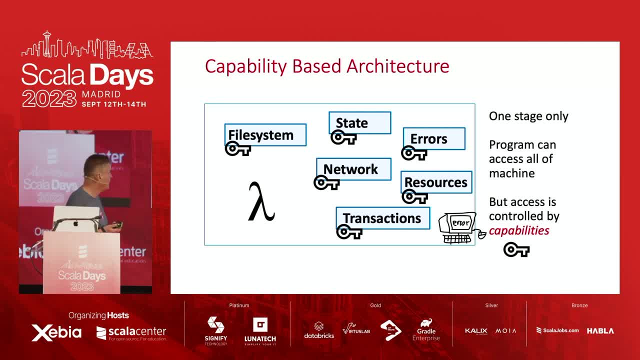 It's supported by the types. It wasn't supported by the types before. So it means that if you have no capability whatsoever, Then Until here you're in the functional world. Functional world means I have no access to resources and defects, but I can sort of bit. 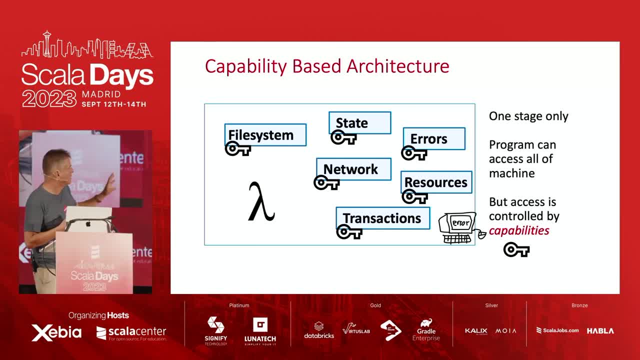 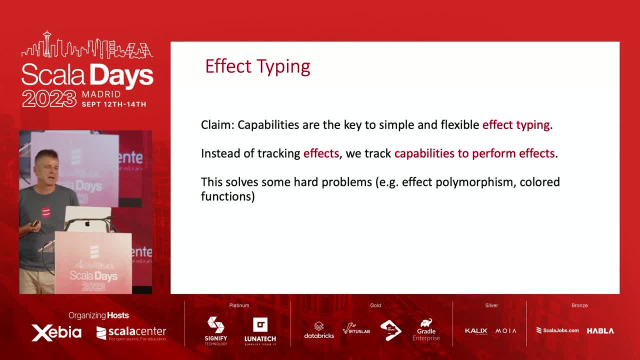 by bit, organically, mix and match, go out there and essentially pick some of these things as as I need them. So the claim is that these capabilities are the key to simple and flexible effect typing. Instead of tracking effects as we do in an effect system, we track the capabilities to. 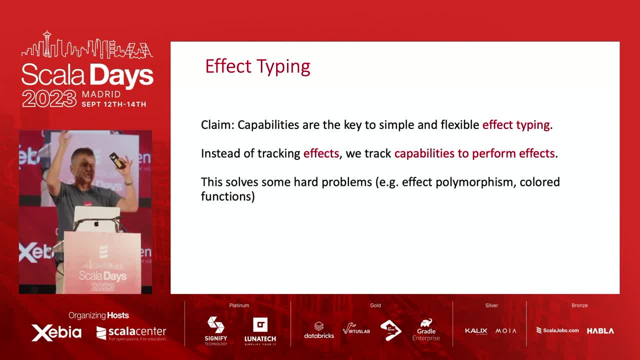 perform effects. So an effect is essentially a part of your result, and a capability to perform an effect is a parameter that you take. We push it from one side of a function to the other And it turns out. I don't have the time to go into this. 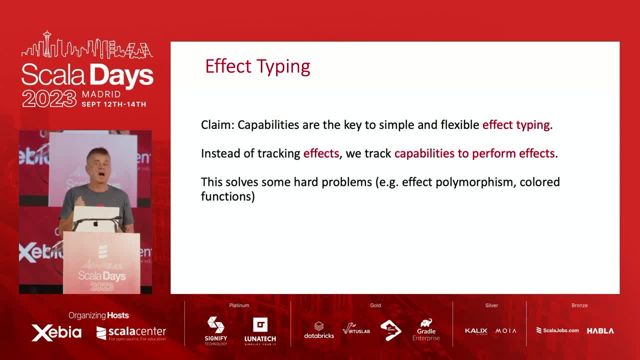 I did that in other talks. This solves some really hard and longstanding problems related to effect polymorphisms and colored functions. So it's actually really good for that, because it solves some of these problems that nobody knew how to attack before. On the other hand, one can ask whether effect typing is actually worth it. 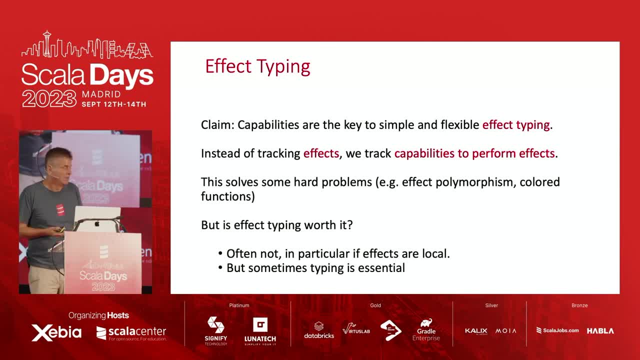 Do we really have to push the type system as far as it will go, And it's true In particular if effects are local? do you really need the assurance that your var is local in a function? A simple code inspection would actually give you that right. 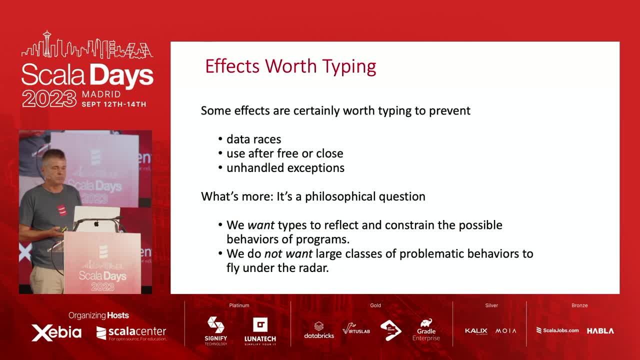 But on the other hand, we've seen, sometimes effect typing is essential. So what do we do? So effects that we definitely want to type is effects that prevent data races. So by tracking them we can avoid data races: fearless concurrency. how rest is? 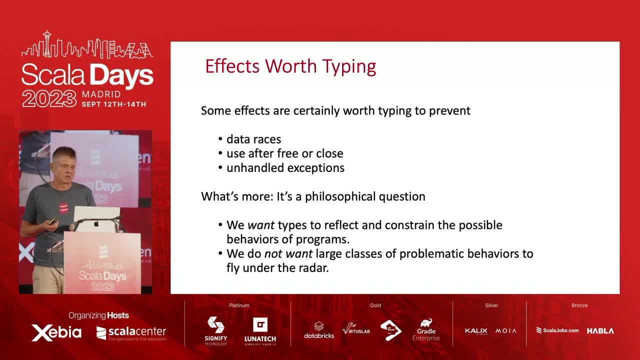 So that's definitely something that would be a quantum leap if we could track that. Other serious errors that could maybe arise only in certain situations are use after free or close unhandled exceptions, things like that, And what's more. I think it's a philosophical question. 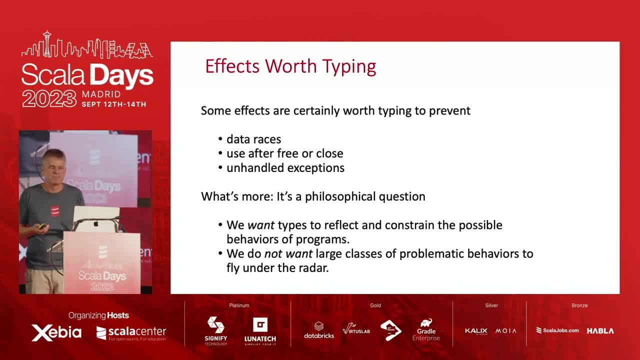 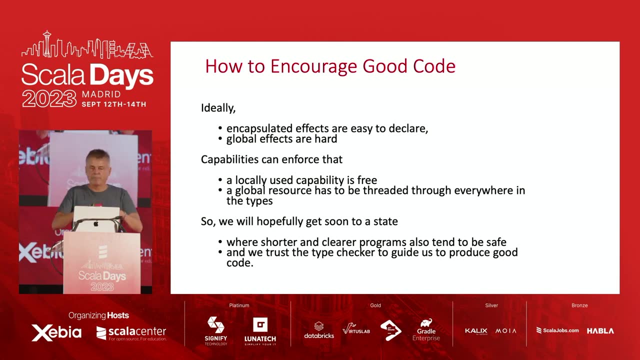 So we want types to reflect and constrain the possible behaviors of programs and we don't want large classes of problematic behavior to fly under the radar. So ideally, my ideal for a language would be a language that makes encapsulated effects- the good kind of effects- very easy to declare, no notational overhead for those, and makes 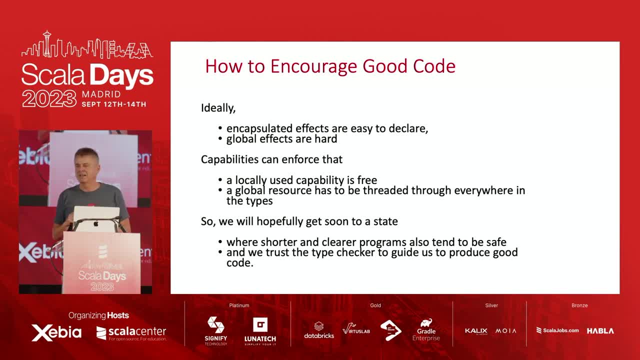 global effects of the like the really bad kind we have seen in the flag translation very, very hard. So it means that if something like that, if you need a global variable like that, you could say, well, you can have it, but you sort of have to add this capability everywhere. 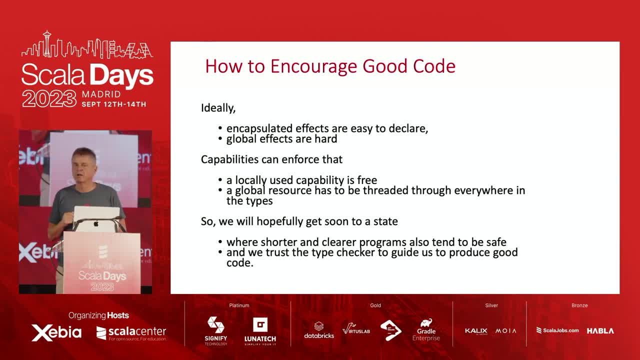 to all your code that you are going to access this global variable And before you're finished, you probably will have changed your architecture and said, no, it's not worth it. Let's keep things simple. The problem right now is that it's too simple to have a global variable. 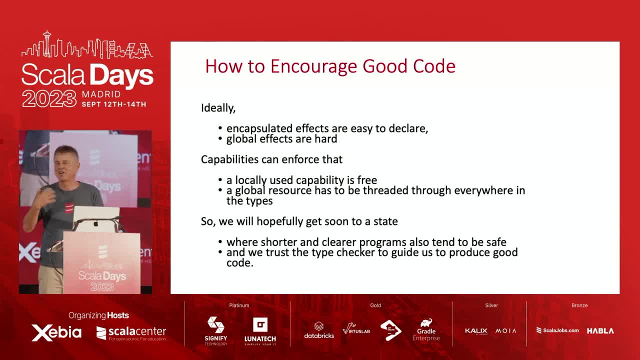 There's no effect whatsoever. You don't see it, See the pain. You don't write the program. It doesn't get reflected in the types. So that means that capabilities should enforce that locally used capability is free and a global resource has to be threaded through everywhere in the types. 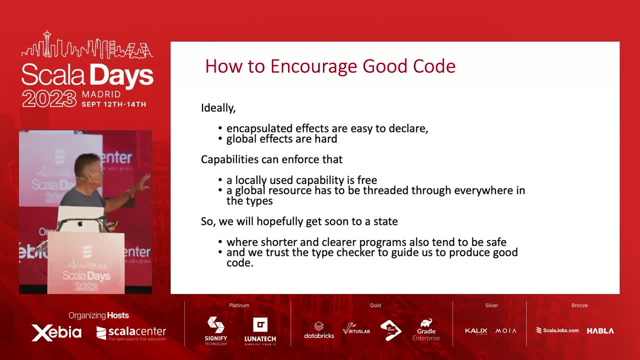 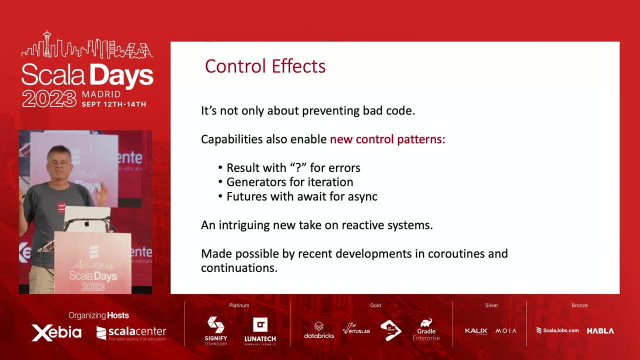 So I believe we're close to getting to a state where shorter and clearer programs also tend to be safe and we trust the type checker to guide us to produce good code, A thing I haven't talked about. Maybe the next talk is Control effects, because it turns out that all this thing with capability is not only 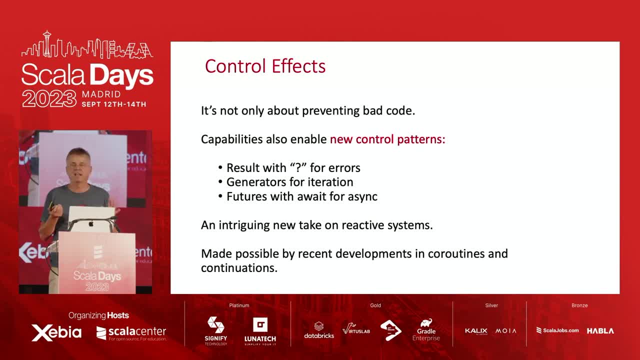 very good at preventing errors. it's also really good at getting new control abstractions in your program. Control abstractions like result with question mark for errors, like what you find in Rust or Swift. generators for iteration, like Python, generators that you find there. futures where? 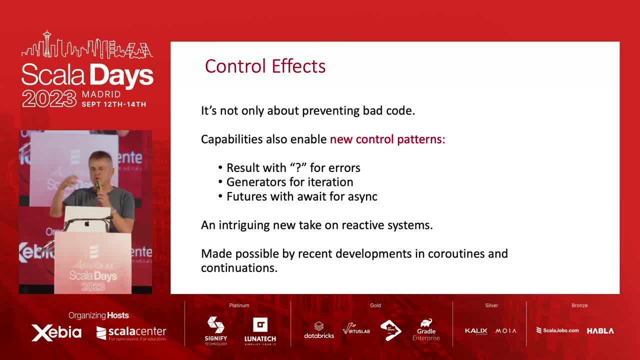 you can actually wait for a future and you don't have to cobble them all together in four expressions and so on. So I believe all together That gives a really intriguing, exciting new take on reactive systems. And what makes it possible underneath is that we are now at a state where essentially something 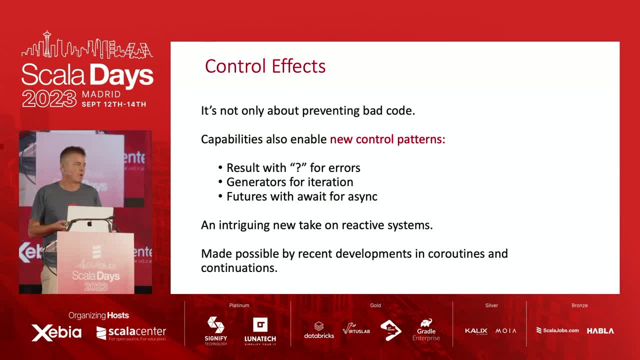 like coroutines and looms, or continuations on which we work in the Scala-native context, are becoming reality, and we can essentially base these systems on these foundations. So what I believe, what Scala should be or where we should go, is instead of going right. 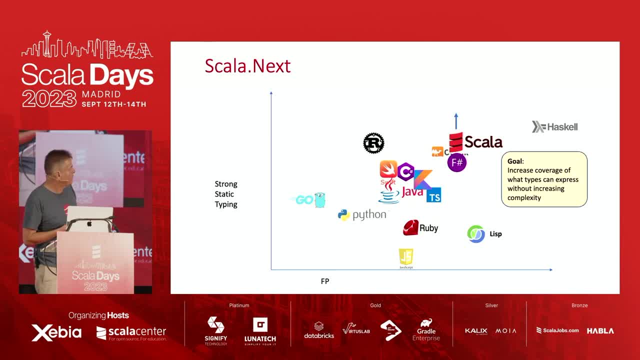 we go up, We go to Exactly, Essentially, more typing, By which I don't mean more intricate type-level programming, not at all. So what I want as a goal is to increase the coverage of what types can express without increasing the complexity. 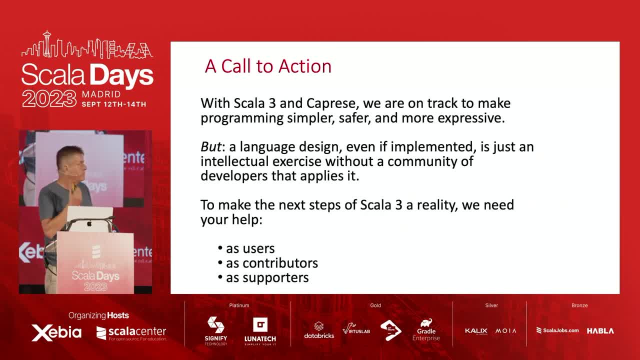 That's essentially the goal where we want to go. So the call to action. So I think we are on a track to make programming simpler, safer and more expressive for Scala 3 and Caprize. But a language design, even if it's implemented, is just an intellectual. 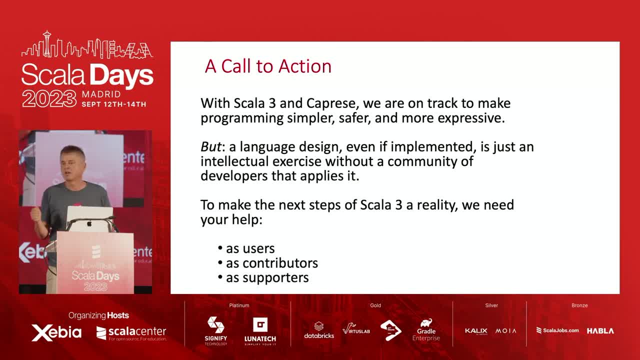 It's not a language design, It's an intellectual exercise without a community of developers that applies it. And that brings me to you. To make the next steps of Scala 3 a reality, we need your help as users, as contributors and as supporters. 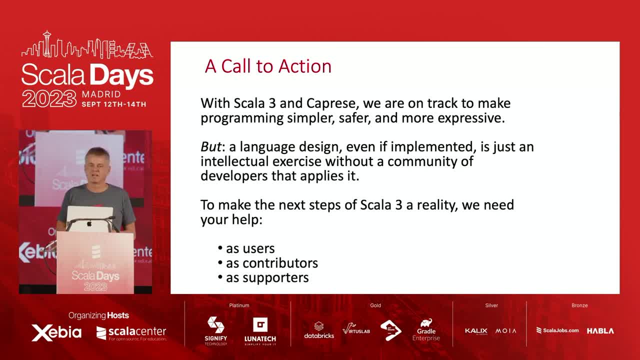 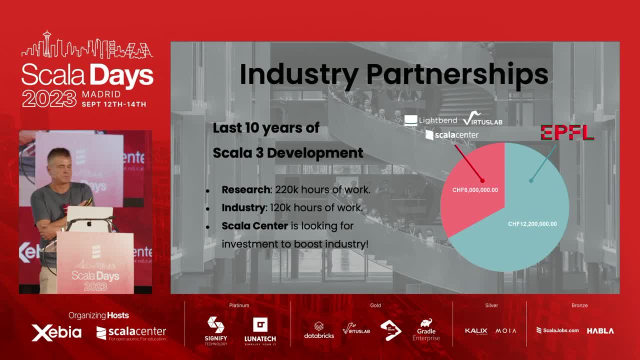 And that brings me to Scala Center, one of the main organizers of this event. So Scala Center has had very fruitful industry partnerships with Lightband, VirtusLab, 47Degrees and so on. But if you look at the total input into, let's say, Scala 3, then it's still largely carried. 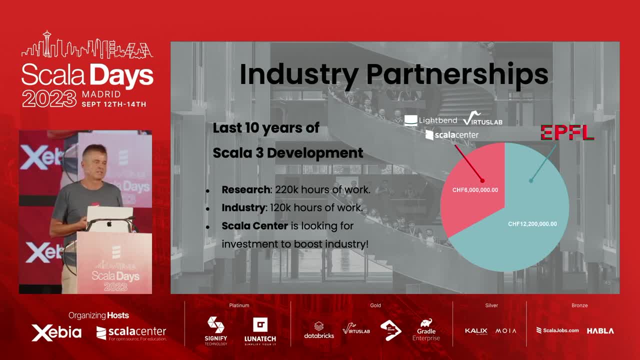 by EPFL, the university and research contracts. And if you want to make Scala 3 a reality in the industrial sense, to really reap the fruits of that, I think we need to sort of make a more even balance of the inputs of 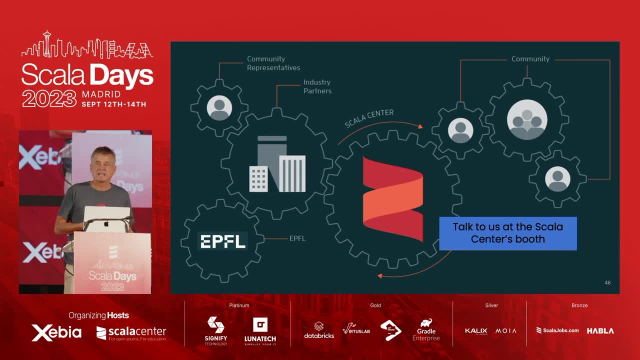 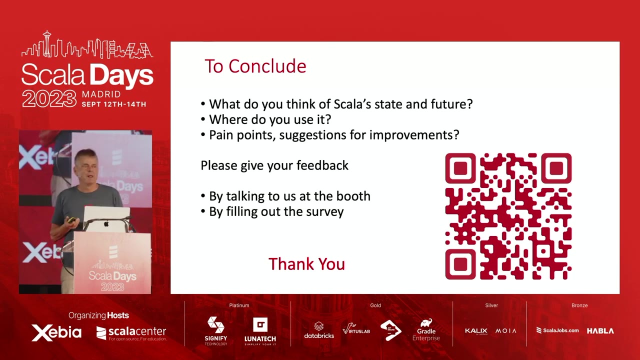 what we can get here. So Scala Center has a booth. If you can help, by whatever means, please talk to us at the Scala Center's booth, which is in the exhibition area. Okay, So I've given you my vision, my spiel. 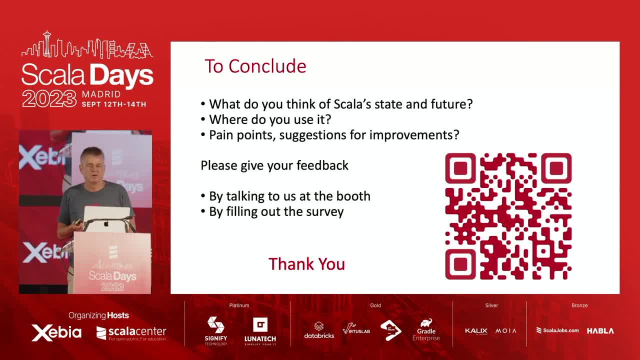 Now it's up to you. I would like to know from you what you think of Scala's state and future. Also quite basic thing: where do you use it currently? Where do you think you might use it in the future? What are your pain points?